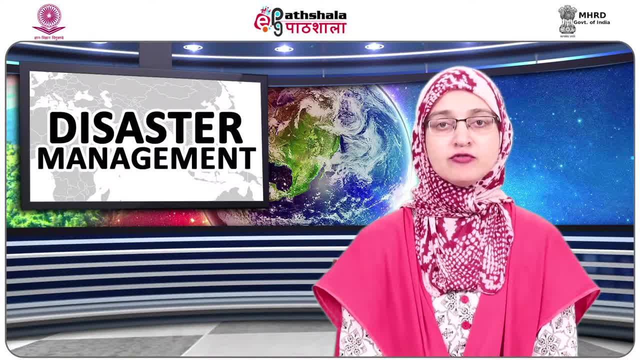 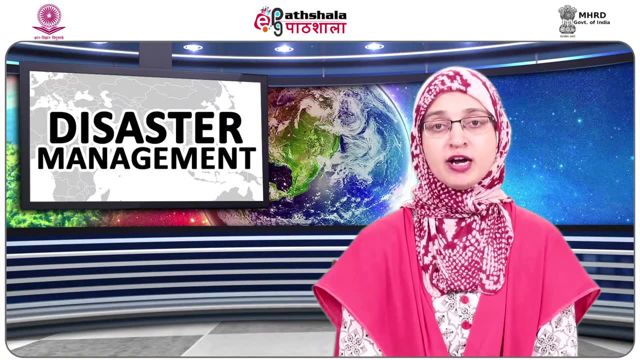 Department, ie IMD, had classified droughts in four broad categories, as under: 1. Meteorological drought over an area is defined as a situation when the seasonal rainfall received over an area is less than 75% of its long-term average ie LTA value. It is further classified as moderate. 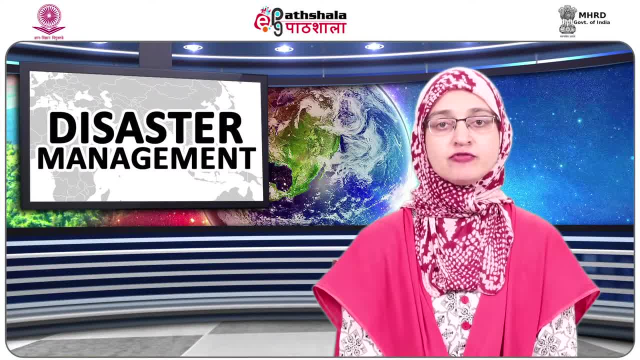 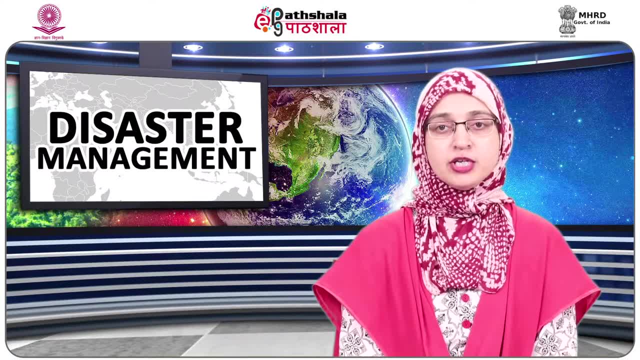 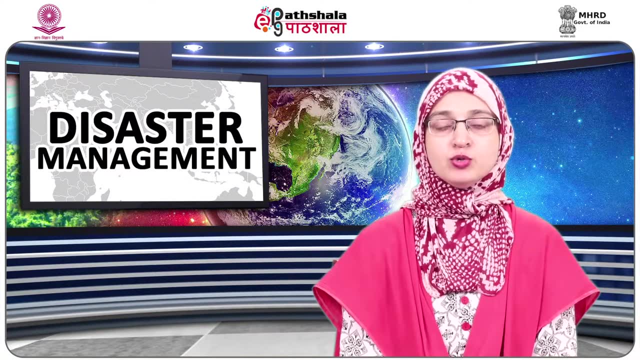 drought if the rainfall deficit is between 26 to 50%, and severe drought when the deficit exceeds 50% of the normal. Major causes of meteorological droughts include lean monsoon, late monsoon, untimely monsoon, prolonged break between two spells. Number two, hydrological drought can be. 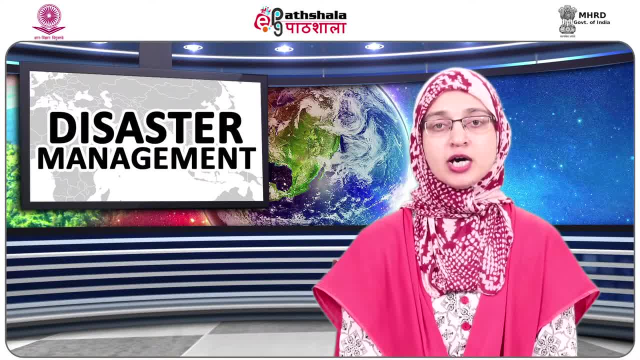 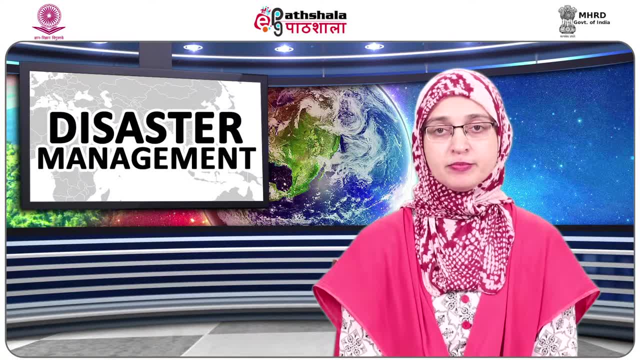 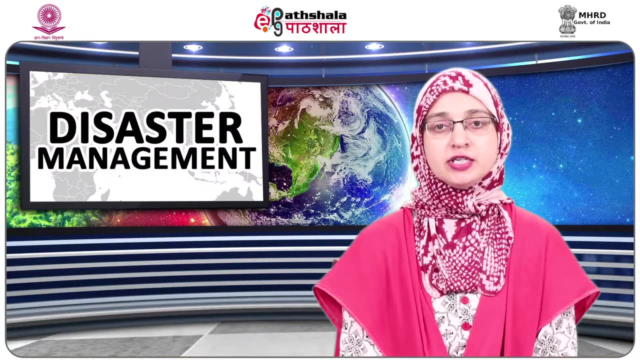 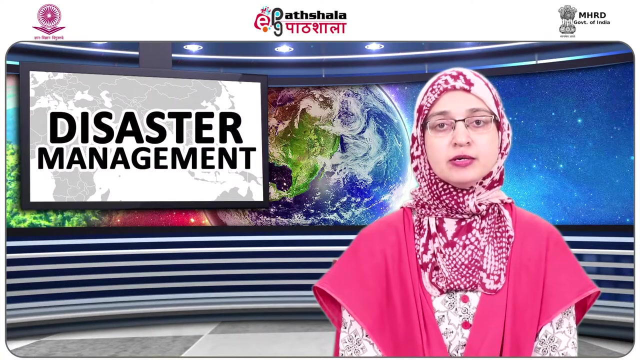 defined as the period during which the stream flows are in advocate to supply starvation. Number three, hydrological drought, can be defined as the period during which the water flow activity decreases with longer periods of time. So adaptation, ероlogical drought can be defined as the period during which the water flow is in vegetable. consumption, such as added water. flow times. Er is again defined as the period during which the water is takenhh. An спорт return on water average is contared with the Robert Stern introduction of hydrological drought. Finally, irrigation is defined as a 사랑 on the enviroment and since it has not been, 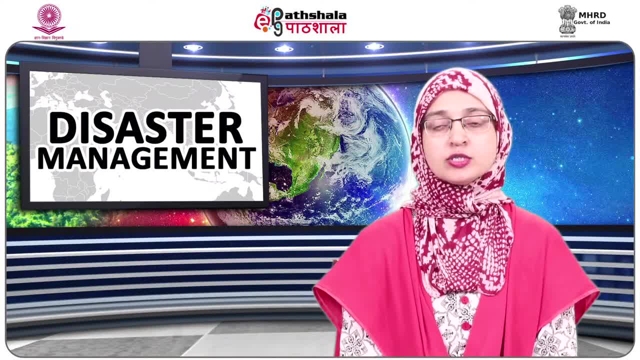 possibly submitted. in the United States the government has strains the guys personally ω educate for healthy crop growth and cause extreme stress and wilting. It is to be noted that agricultural drought is relative, as drought condition for rice cultivation is different than the drought condition for millet cultivation. 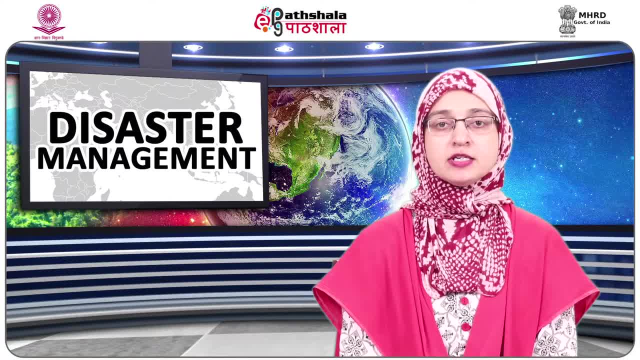 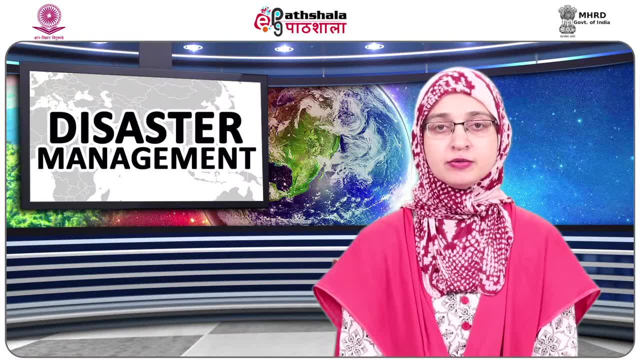 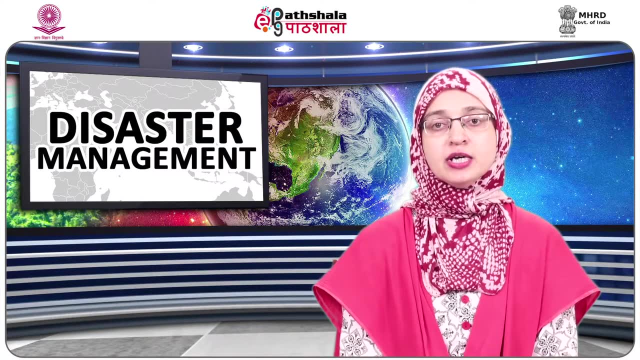 4. Socio-economic drought occurs as a result of the above three types. Abnormal water shortage affects all aspects of established economy of a region. This in turn adversely affects the social fabric of the society, creating unemployment, migration, discontent and various other problems in the society. 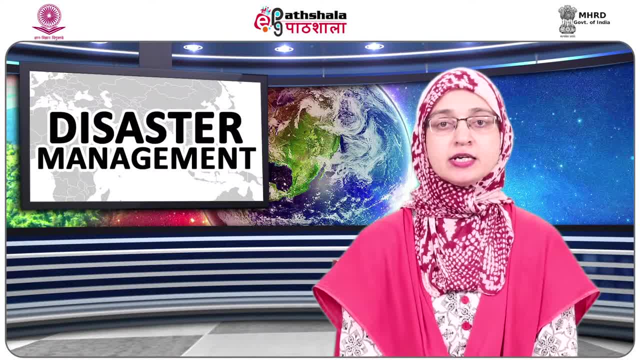 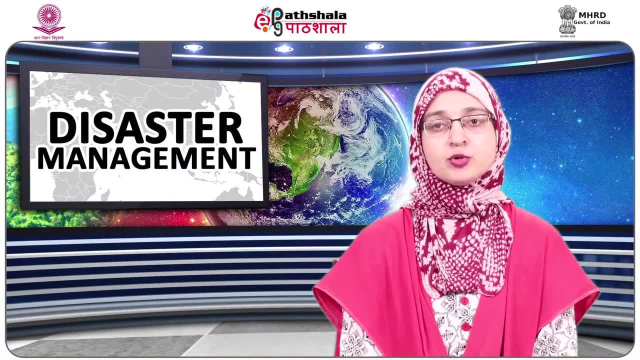 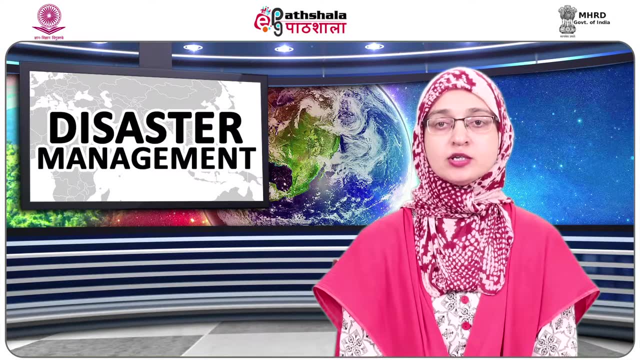 Apart from the above types, there can be one more category, that is, ecological drought. that is considered as a condition where environmental degradation reduces the productivity of the natural ecosystem significantly. In many cases, more than one reason contribute to the problem. 1. Famines. 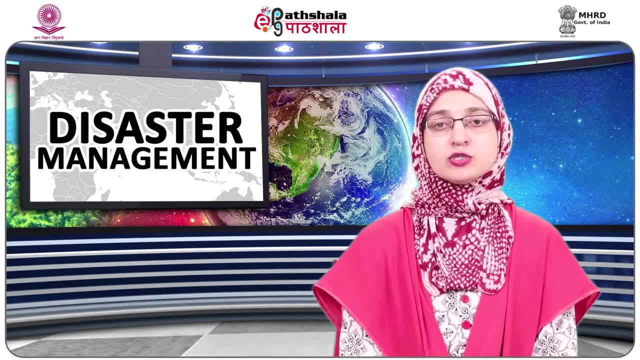 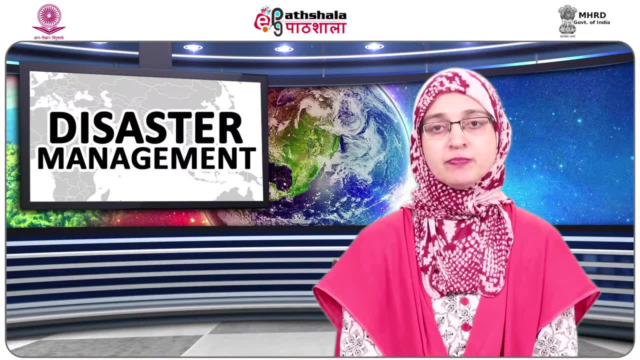 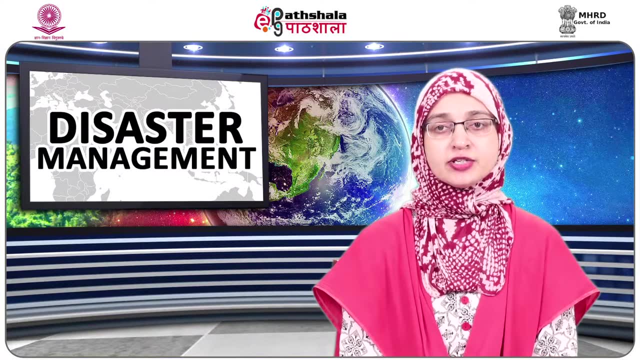 Famines and droughts are often interlinked, though they are two distinct phenomena, often occurring in a cause-effect relationship, with famine succeeding a prolonged drought period. Famine is a severe scenario where extreme scarcity of food is experienced, leading to mass malnutrition, starvation, increased mortality and epidemic scare. 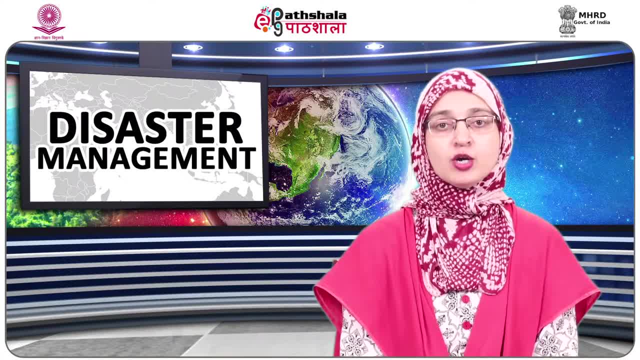 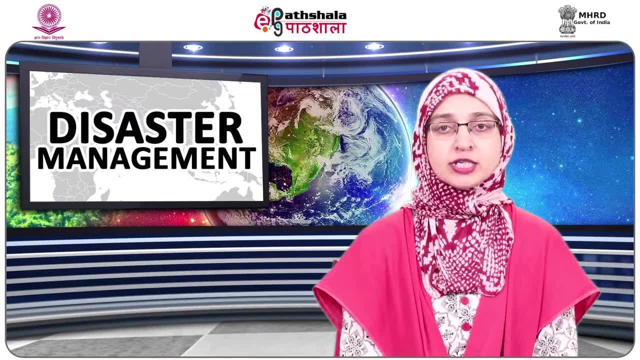 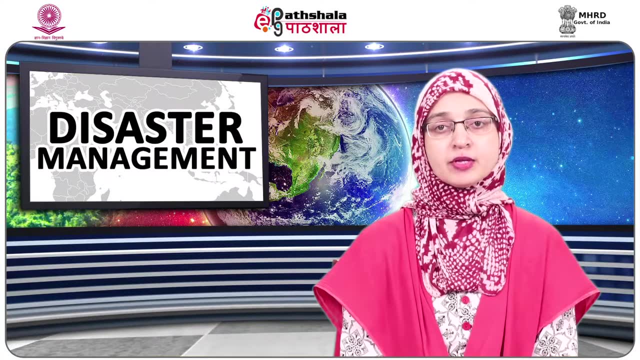 It may result from droughts leading to crop failure, low food availability or poor access to food, But more often, rather than actual food scarcity, socio-economic complexities may also play a major role in the occurrence of famines. 2. Desertification- 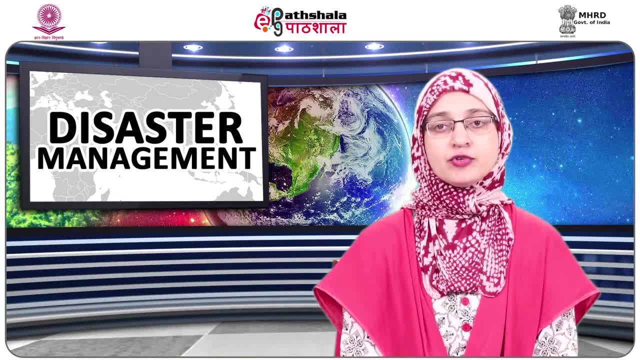 It is a condition which often occurs as a result of extreme soil water deficit. It results in the degradation of land, loss of water bodies, flora and fauna. 3. Desertification- Citing an example, Sahel region in Africa is characterized by high temperature, hot. 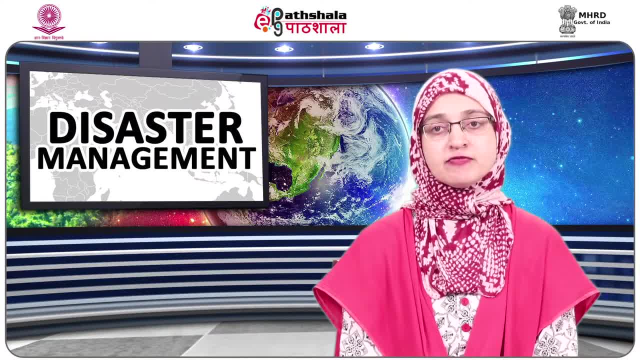 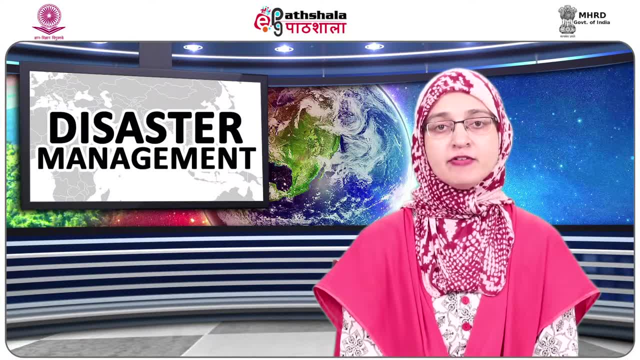 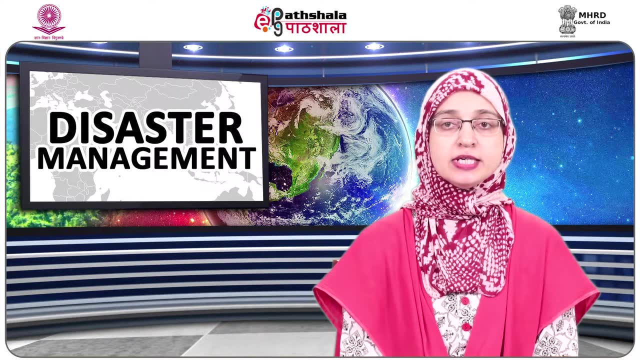 climate and very low rainfall, which created massive desertification, losing significant amount of productive and to deserts. This has affected about 6 million citizens residing in the area, according to UNC 2016.. 4. Impact of droughts: Now, impacts of droughts. 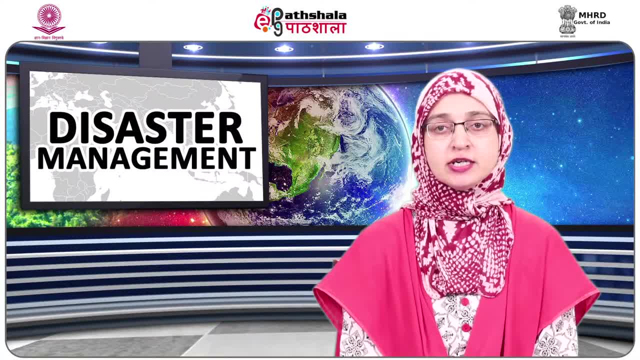 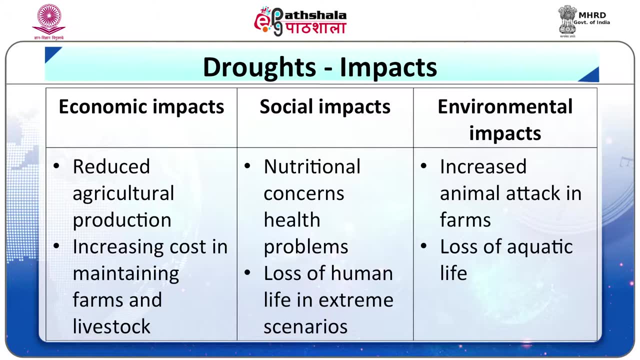 1. Economic impacts. Drought impacts are often multifaceted and non-linear due to the complexities associated with their occurrence. They can be classified into three major categories: 1. Economic impacts: These include the aspects which directly or indirectly impact the well-being of a person. 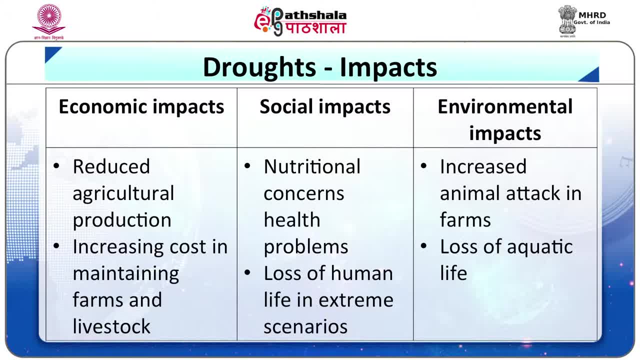 of the society. The main factors of economic impacts are: a- Reduced agricultural production, leading to reduced harvest and thereby reduction in the crop yield. b- Increased cost of farm maintenance due to the additional cost of water provisions and other resources to the farm products, including the reduced usage of fertilizers or chemicals. 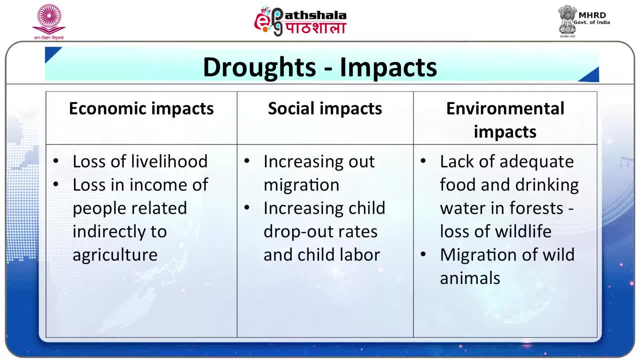 leading to lesser output. c- Loss of livelihood for marginal farm workers. d- Increasing cost of maintaining livestock due to shortage of fodder and drinking water. Often livestock are subjected to droughts. They are often sold to earn extra income during lean months or drought situations. 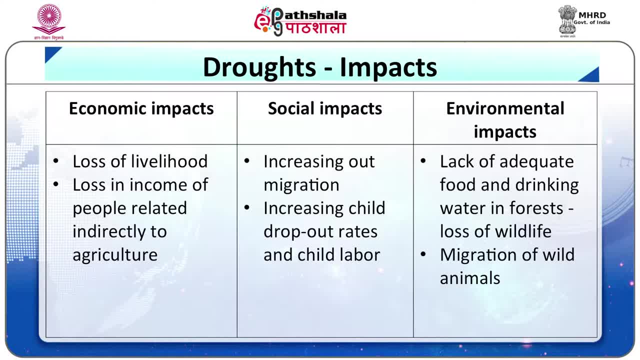 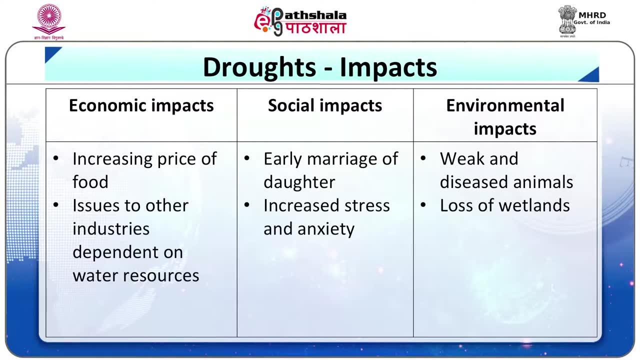 e. Loss in income of people relating to agricultural practices, like agricultural transporters, pesticides and fertilizers retailers, etc. f. Increase in the price of food production due to shortage of supply. g- Economic impacts on other industries dependent on water resources like hydrogen oxygen. 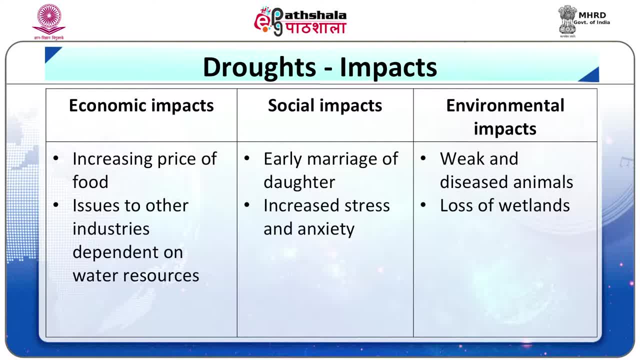 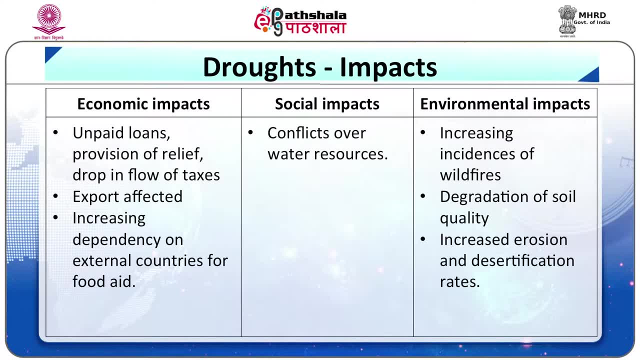 like hydroelectric generation companies, waterways operators and transporters, tour operators, etc. Number H: unpaid loans, provision of relief to the affected and the subsequent burden on government exchequer. Number I: in severe cases, export is affected significantly and increasing dependency on external countries. 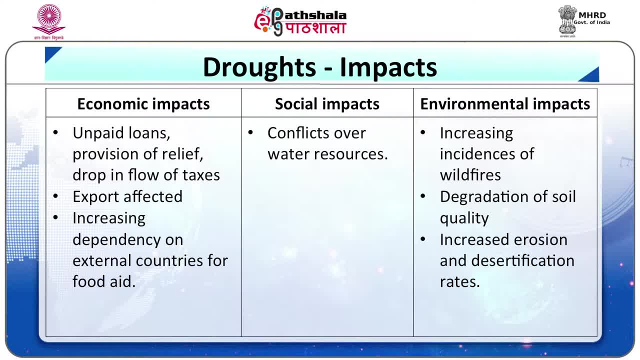 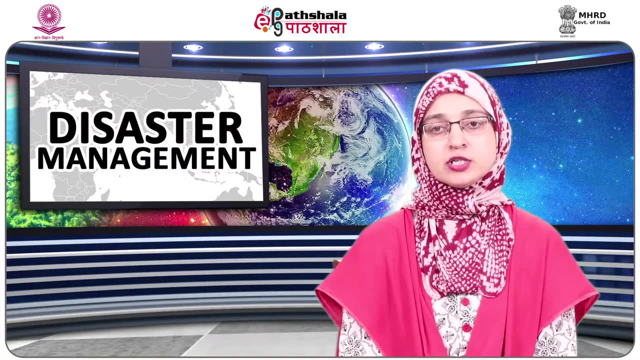 for food aid or import may be required, endangering the food's severity of a nation. Number J: flow of taxes. Now two social impacts: Drought has serious impacts on health and social safety. Lack of water resources often leads to gradual conditions of water deficit. 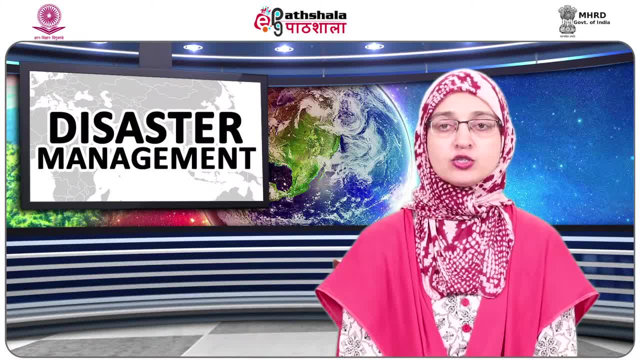 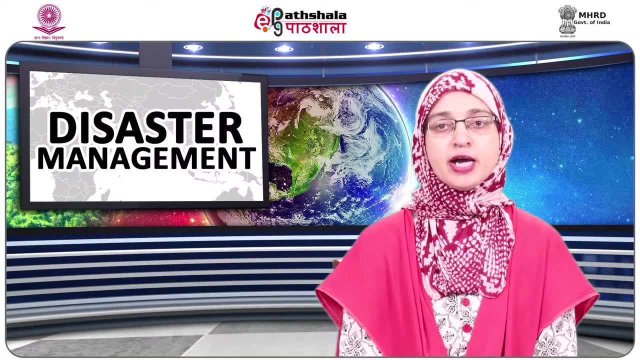 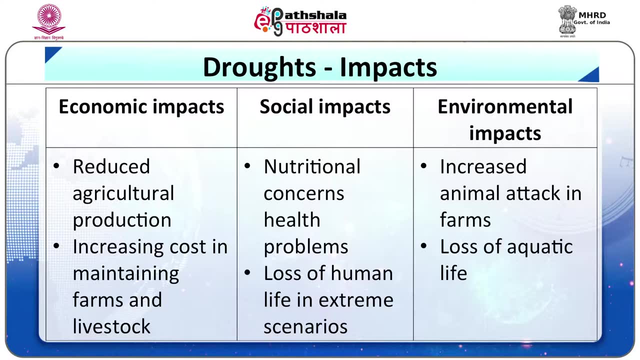 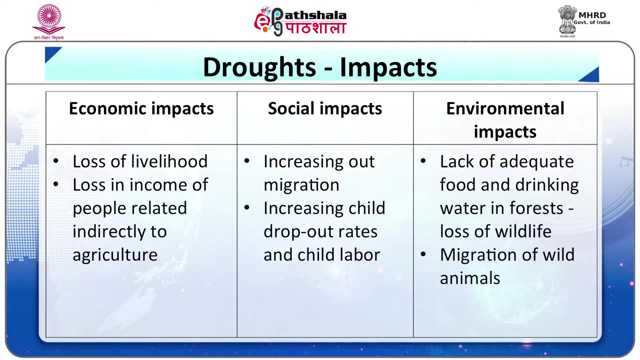 and its extreme form results in long-drawn conflicts. It also affects psychological well-being significantly. The major impacts of droughts include: Number A: nutritional concerns due to poor quality diet and allied health problems- loss of human lives in the extreme scenario. Number B: increasing out-migration in search of alternate jobs to urban areas. 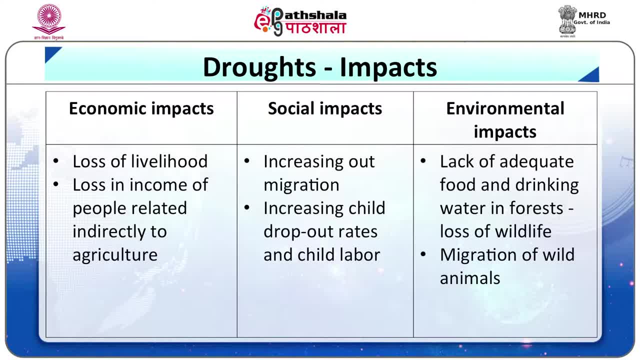 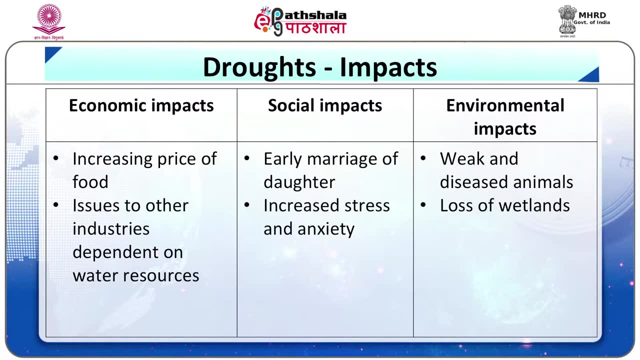 which in turn increase the vulnerability of migrants as they settle squirt in risky environments. Number C: increasing child drop-out rates and child labor. Number D: early marriage of daughters to reduce financial burden and the linking of non-marriage of daughters to the drought occurrence. 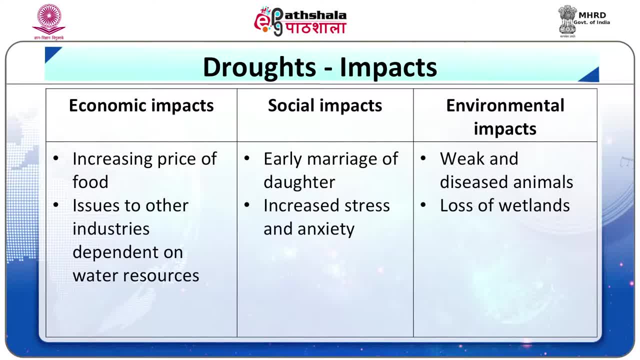 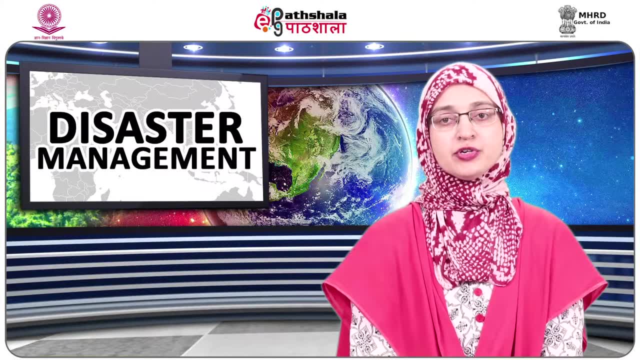 Number E: increased stress and anxiety resulting in increasing incidence of farmer suicide. Number F: conflicts over water resources. Number 3, environmental impacts. Number D: environmental impacts. Number C: environmental impacts. The most severe impact of drought is upon the environmental resources. 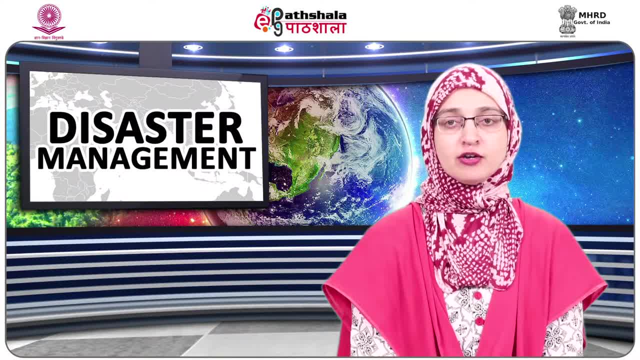 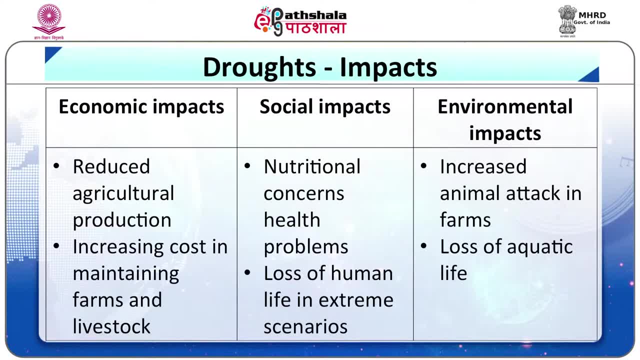 Often, drought results in extensive damage to flora and fauna of a region. The significant impacts include: Number A: increased animal attacks in farm areas due to lack of food in their own habitats. Number B: loss or destruction of fishes and aquatic organisms. Number C: lack of adequate food and drinking water in forests. 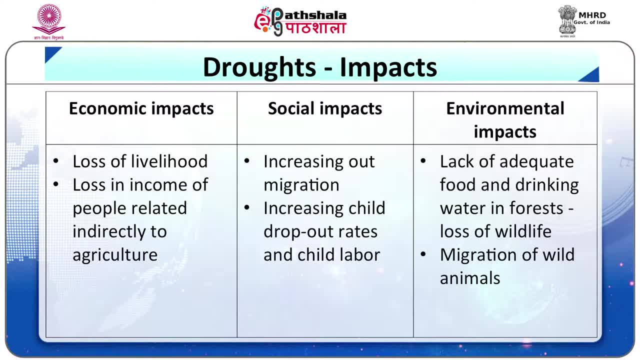 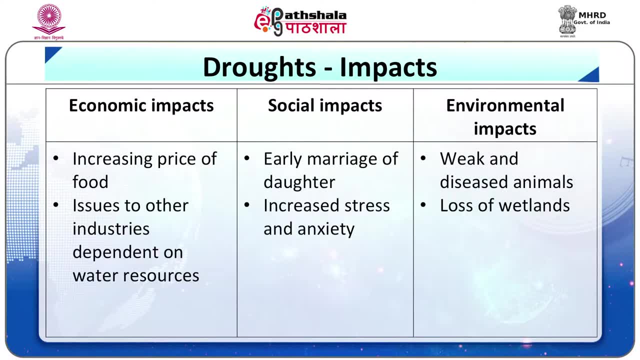 and, in extreme cases, resulting in loss of wildlife. Number D: migration of wild animals, thereby increasing human-animal conflicts. Number E: weak and diseased animals. Number F: loss of wetlands and increasing incidences of wildfires. Number G: degradation of soil quality and soil productivity. 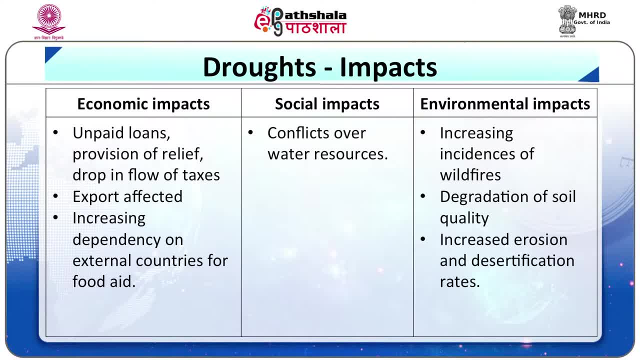 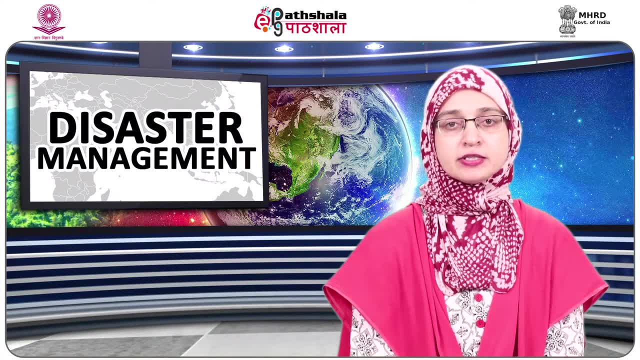 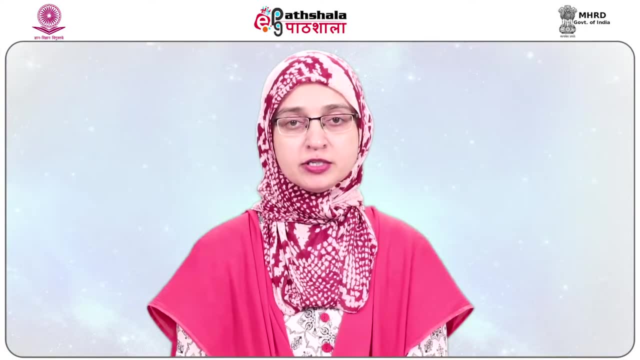 Number H: increased erosion and desertification rates. These direct impacts have multiplied and results in the indirect impacts that are often diffused and complicated to be gauged appropriately. In the historical past, droughts and famines have often been interlinked. 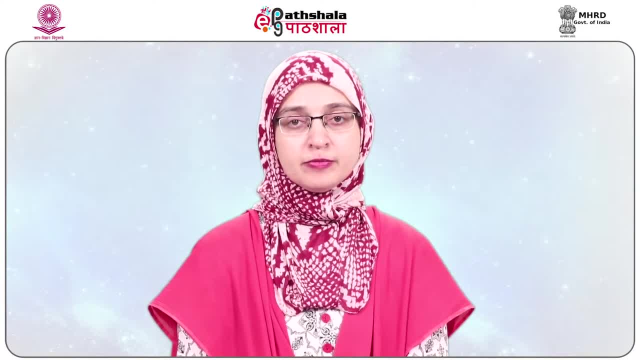 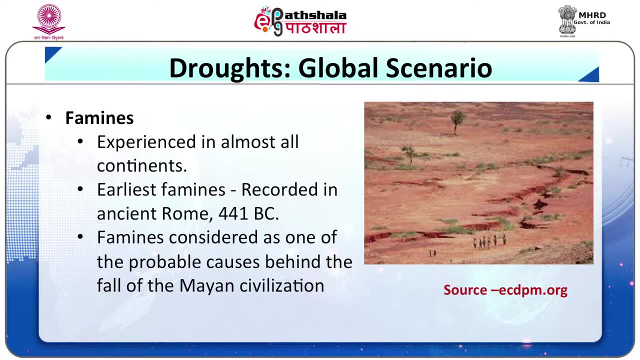 and the terms have been used synonymously. Famines have been experienced in almost all the continents. One of the earliest famines recorded was in ancient Rome in 441 BC. Famines are considered to be the most common and most common species of animals in the world. 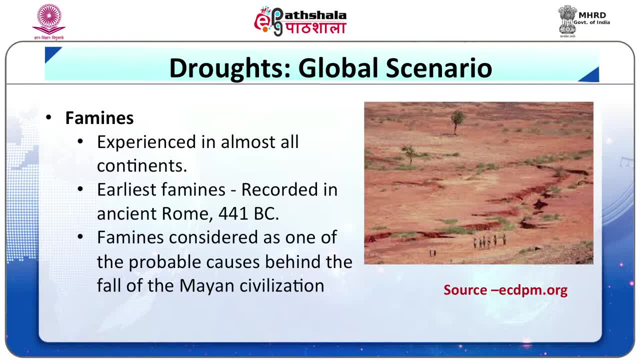 Famines are considered to be the most common species of animals in the world. Famines are considered as one of the probable reasons behind the fall of the Mayan civilization of Mesoamerica as one of the probable reasons behind the fall of the Mayan civilization of Mesoamerica. 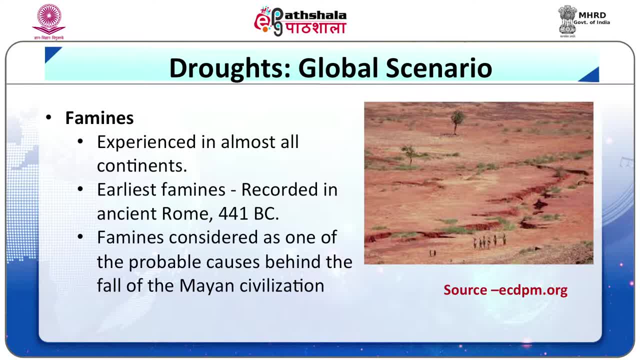 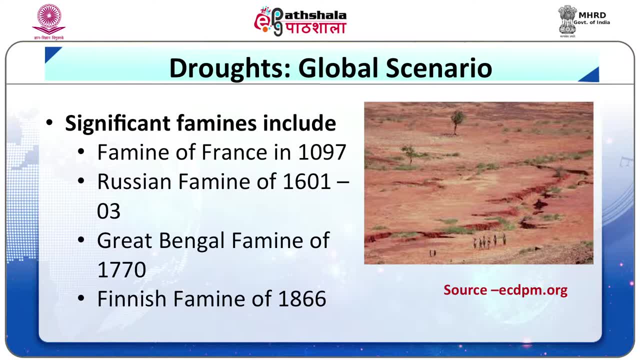 that is, Mexico and Central America in 800 to 1000 AD. Other significant famines include Famine of France in 1097,. Russian Famine of 1601 to 1603,. Russian Famine of 1601 to 1603,. 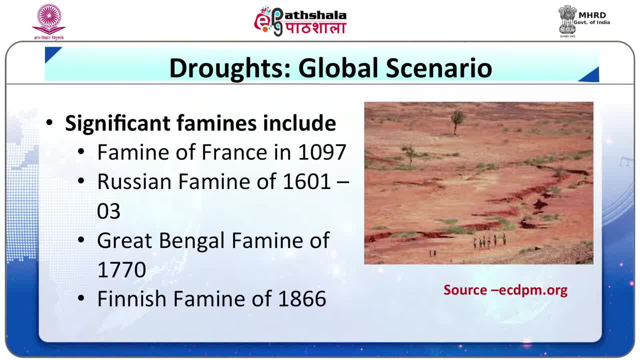 Great Bengal Famine of 1770,. Great Bengal Famine of 1770,. Finnish Famine of 1866, etc. Finnish Famine of 1866, etc. Famines persisted in the region of Europe, but not in the region of Europe. 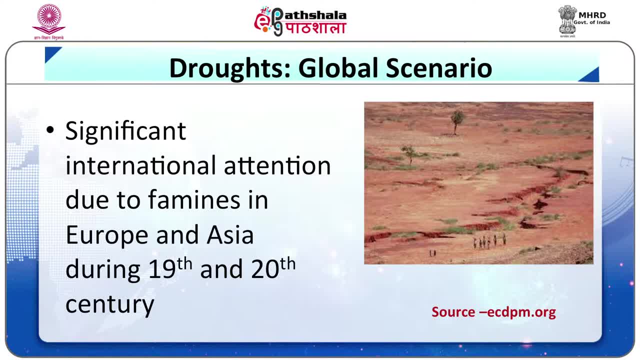 Famines persisted in the region of Europe, but not in the region of Europe. Famines persisted in the region of Europe, but not in the region of Europe. Famines persisted in the region of Europe, but not in the region of Asia. 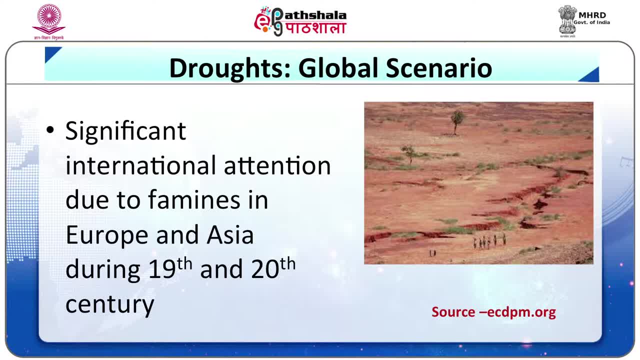 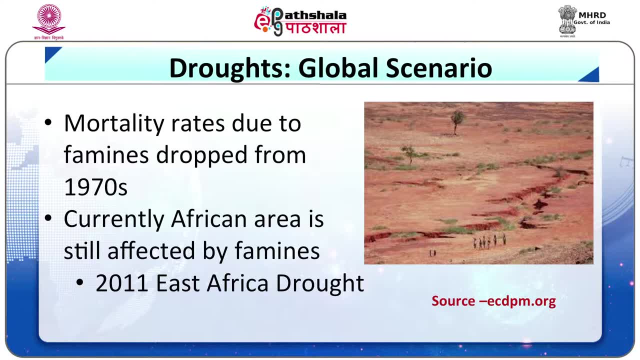 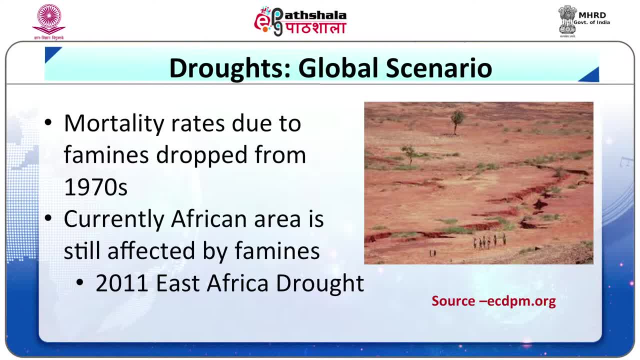 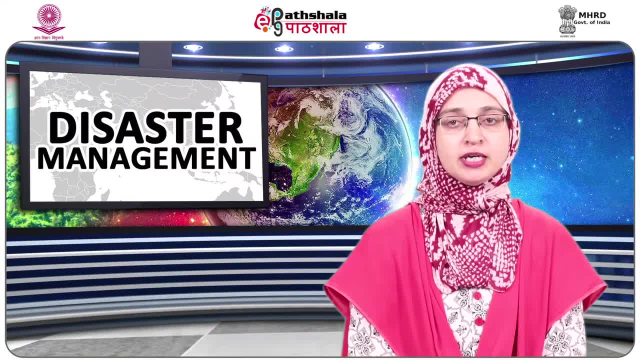 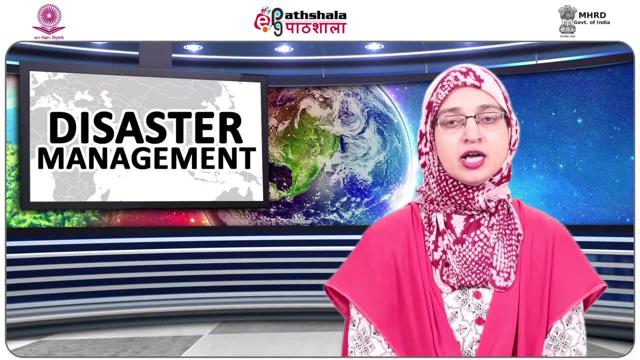 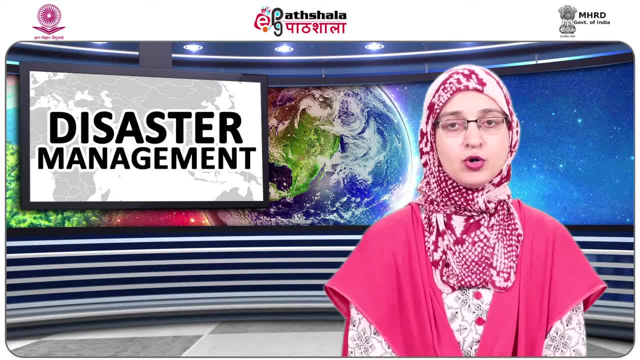 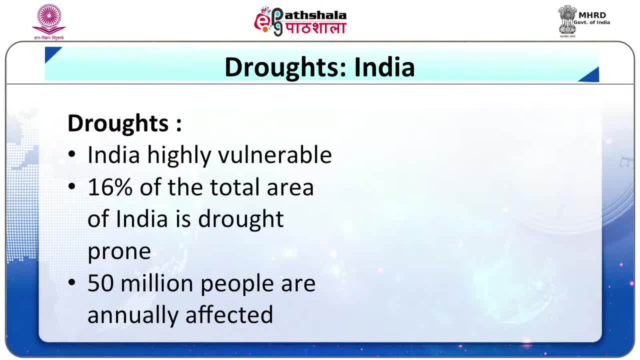 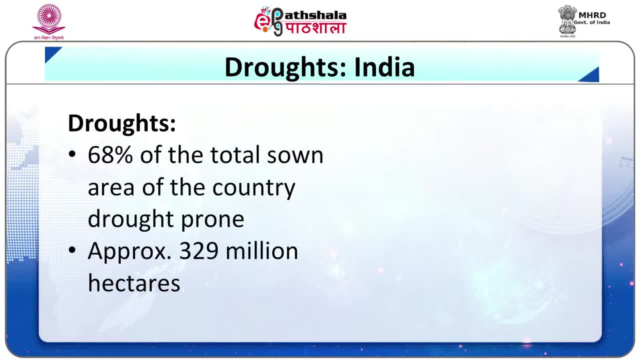 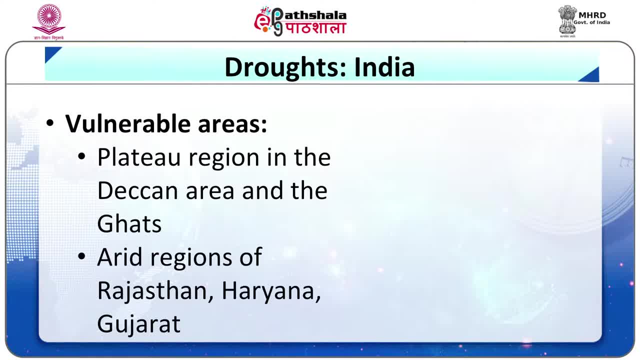 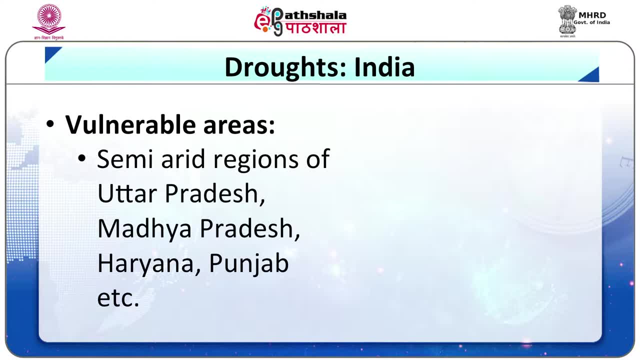 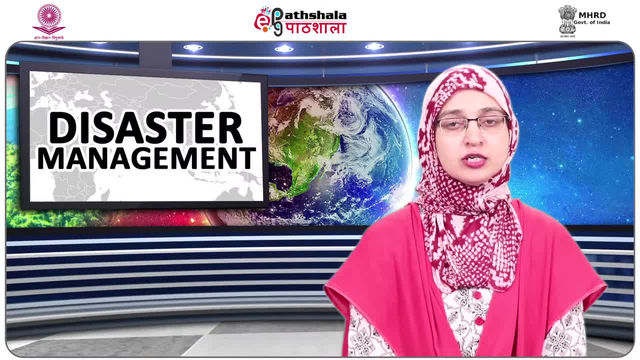 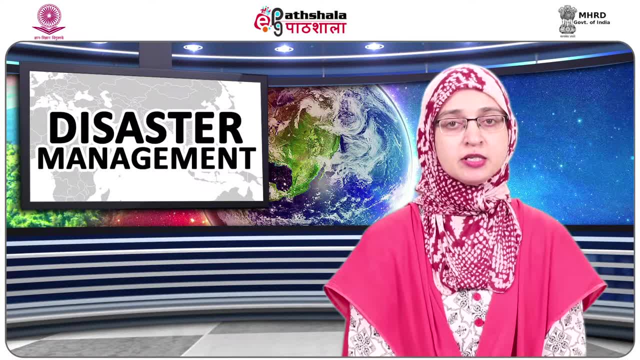 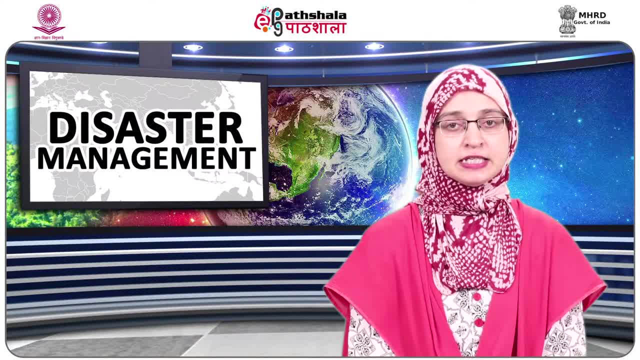 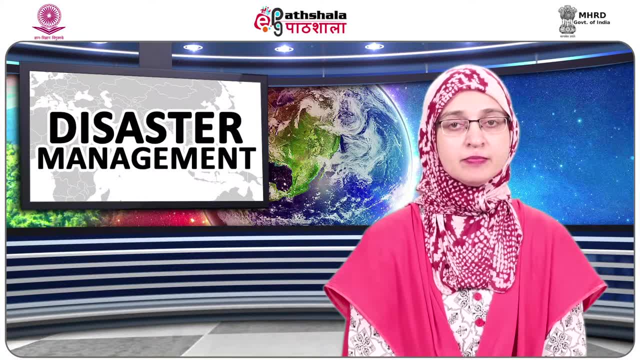 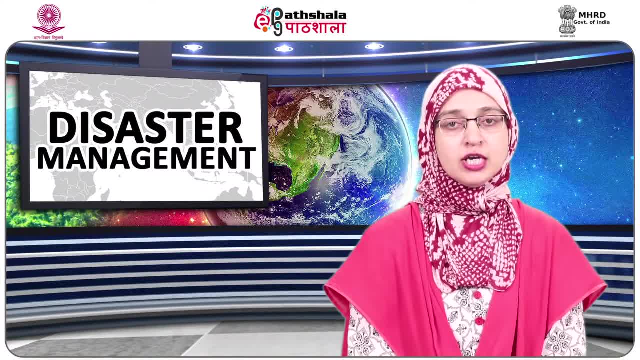 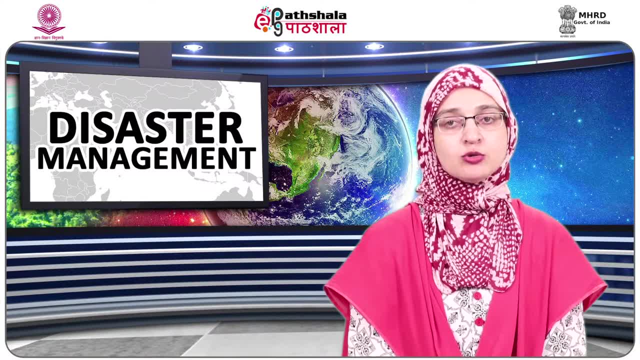 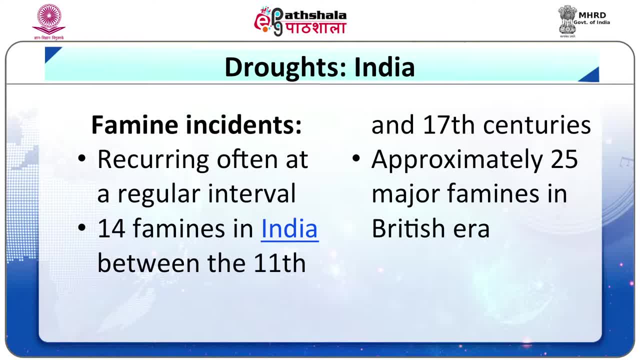 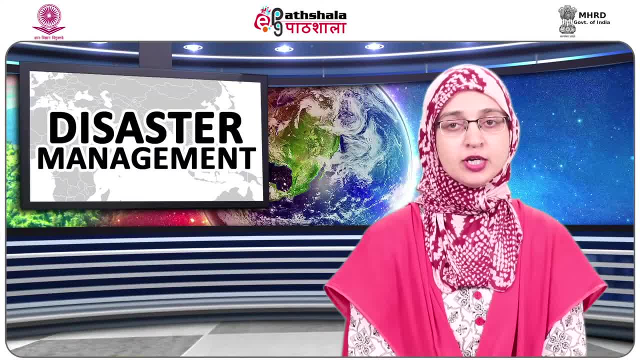 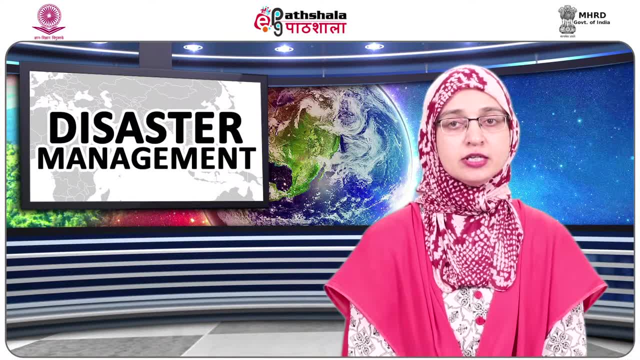 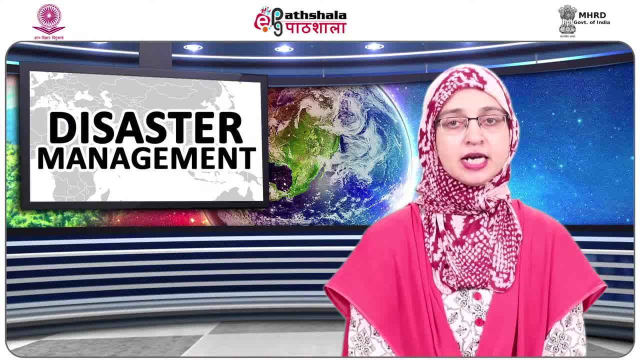 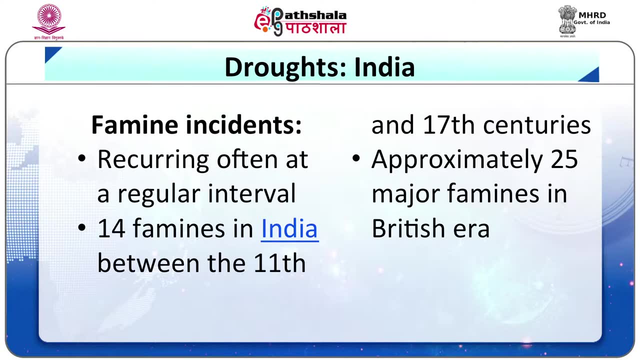 were depopulated. Famine in Deccan killed at least 2 million people in 1702 to 1704.. The famines during the earlier period were highly localized. During the British era, approximately 25 major famines occurred across India. 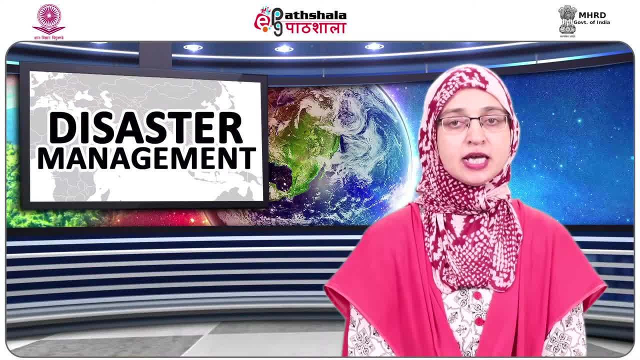 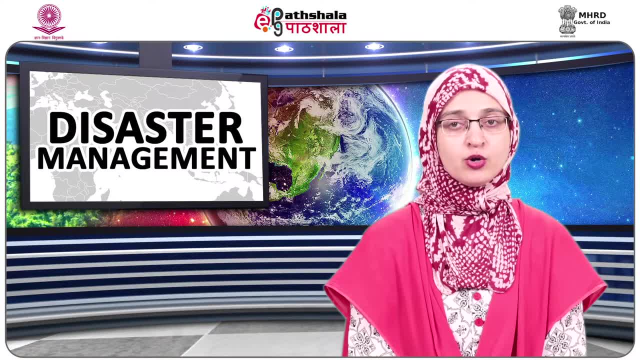 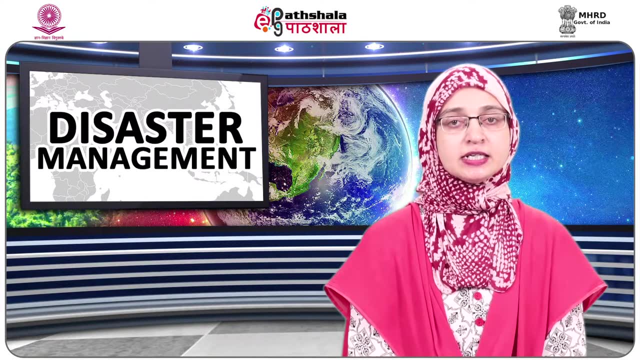 The first Bengal famine of 1770 is estimated to have taken around 10 million lives, which equaled one-third of the population of Bengal. In the famines of 1876 to 1878 and 1899 to 1900, again millions perished. 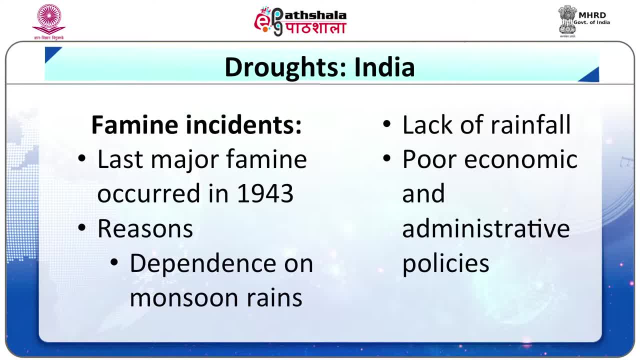 The last major famine occurred in 1943, during the World War, killing an estimated 2.1 million. The famines were resulted due to the lack of rainfall and poor economic and administrative policy. The famines were probably because of the lack of food. 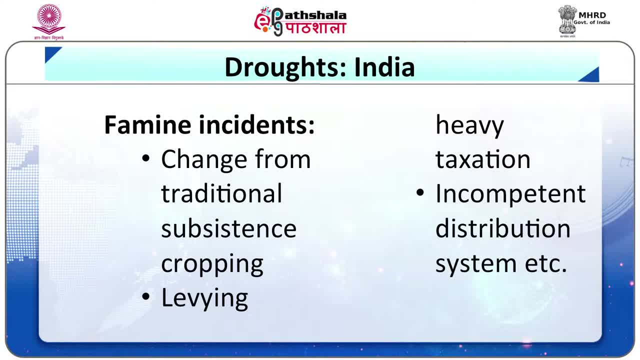 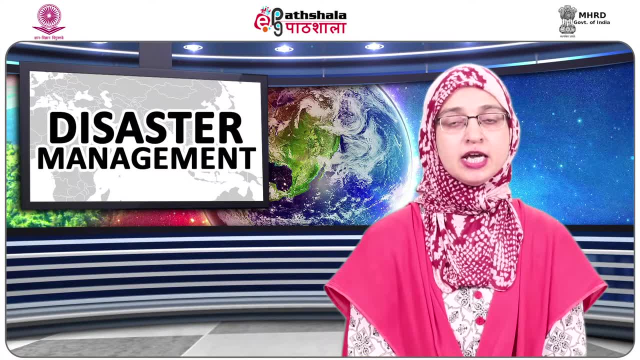 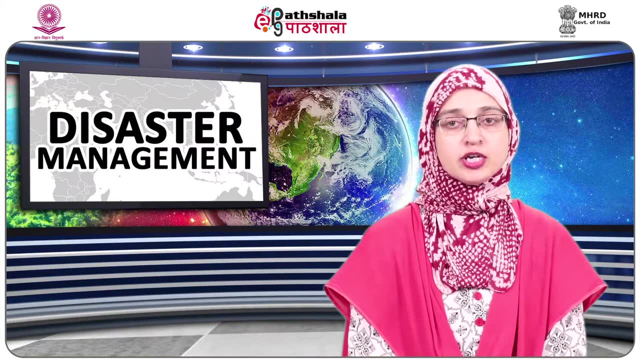 The famines suffered from the change of traditional subsistence cropping. levying heavy taxation, incompetent distribution system and other issues led to increased price of food, which resulted in the tragic drought incidents from the 19th century. Now, Unit 3, Drought: Institutional Mechanism. 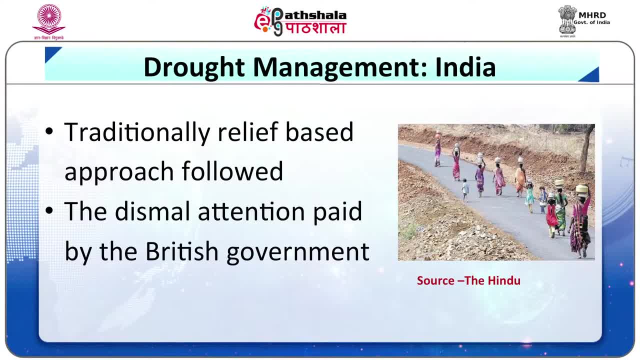 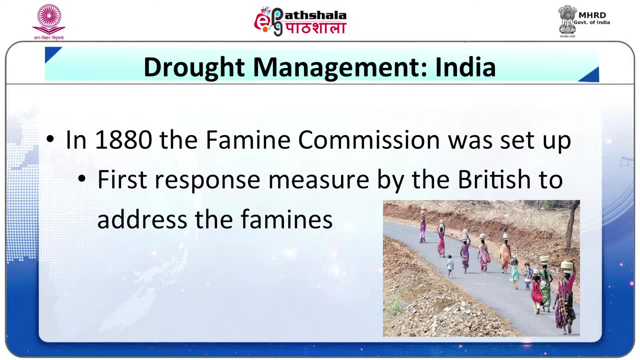 It is historical background. Traditionally, a relief based approach was followed in India for addressing drought drought. The dismal attention paid by the British government during initial famines was highly criticized. In 1880, the Famine Commission was set up as the first response measure taken by 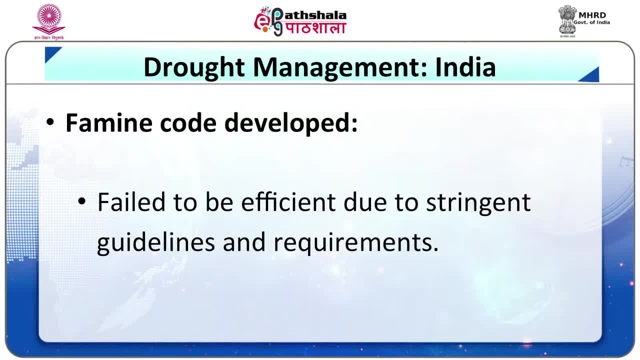 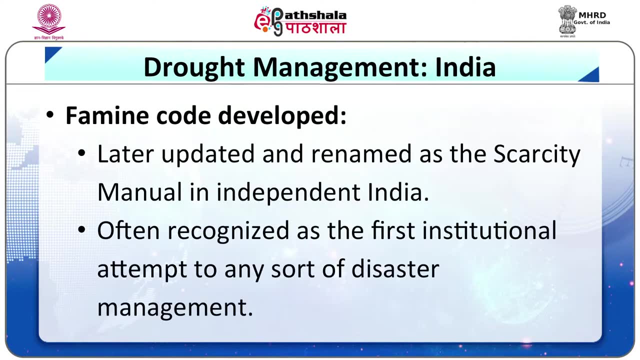 Britishers to address the famines, The Famine Code was developed, but it failed to be efficient due to stringent guidelines and requirements which often required one to wait till the drought actually occurs to take any action. It was later updated and renamed as the Scarcity Manual in the 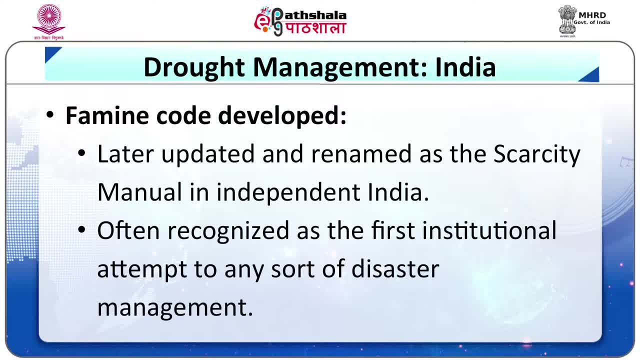 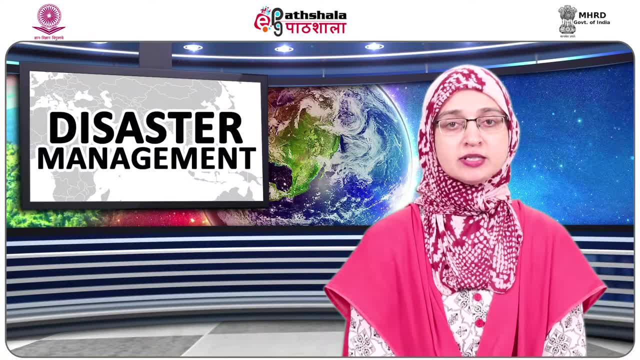 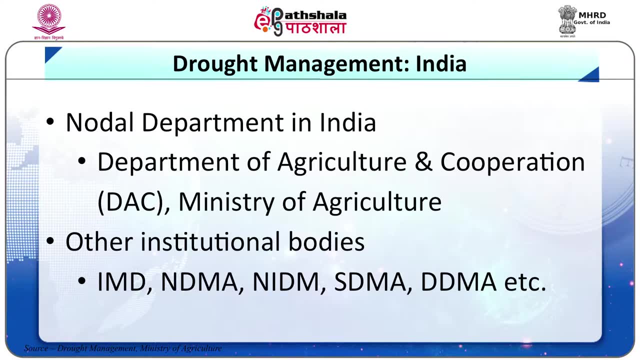 Independent India. Often this is recognized as the first institutional attempt for management of disasters. Now existing institutional mechanism to address droughts in India. The nodal department to address drought in India is the Department of Agriculture and Cooperation, that is, DAC and the Department of Agriculture and Cooperation. The Department of Agriculture and Cooperation. 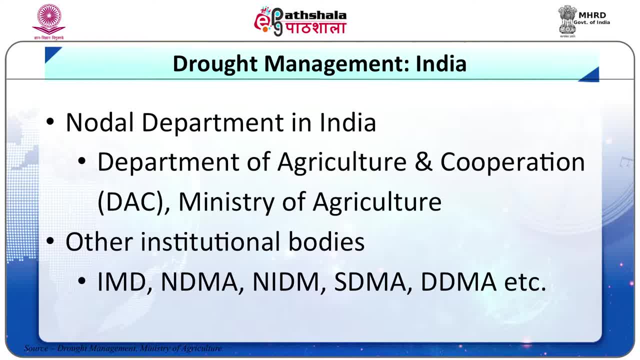 is the Department of Agriculture and Cooperation. The Department of Agriculture and Cooperation is the under the Ministry of Agriculture Government of India. The other institutional bodies functioning in the sector are NDMA, NIDM, SDMA, DDMA and IMD, etc. Two significant guidelines that were 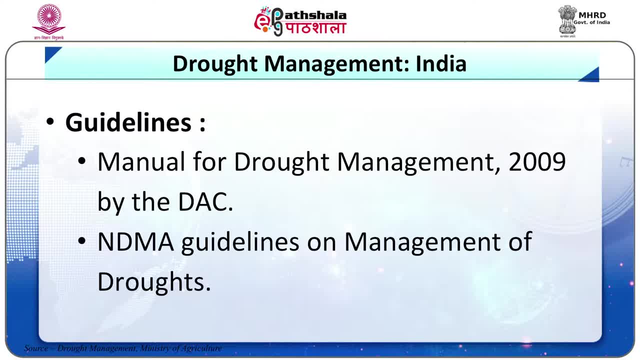 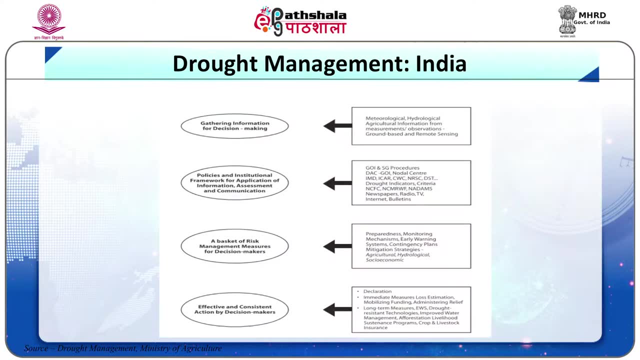 released by the Indian government to address droughts are: number one: Manual for Drought Management 2009 by the DAC. Number two: NDMA Guidelines on the Management of Droughts. Figure one shows drought management strategy. The key components of the guidelines are as follows. 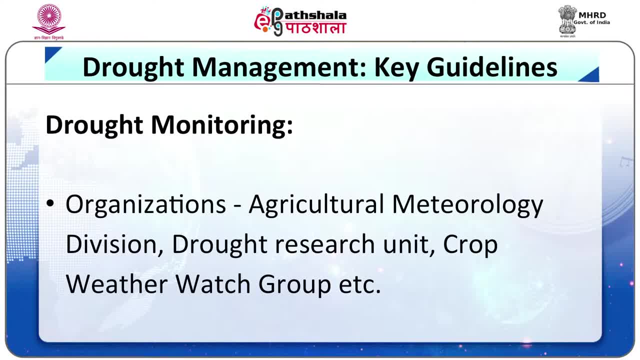 Number A Drought Monitoring. It is carried out through different institutions, which include Agricultural Meteorology Division, Drought Research Unit, National Center for Medium-Range Weather Forecasting and other institutes under IMD, Ministry of Earth Sciences, CROF. 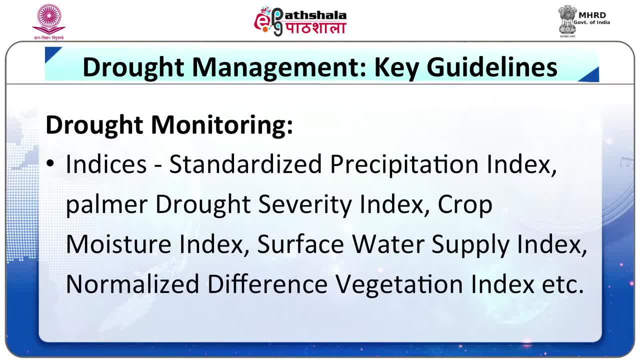 Weather Watch Group, etc. Multiple indices are used for drought monitoring, which include Standardized Precipitation Index, Palmer Drought Severity Index, Crop Moisture Index, Surface Water Supply Index, Normalized Difference Vegetation Index, etc. Number B: Drought. 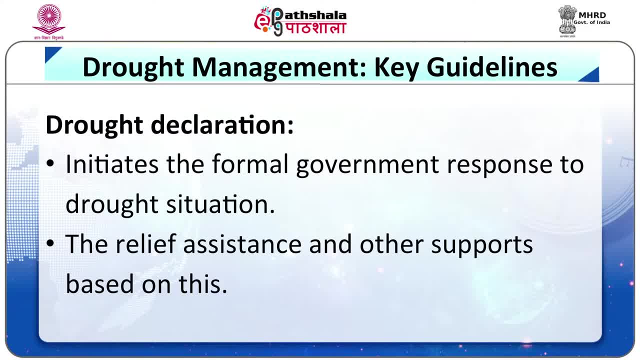 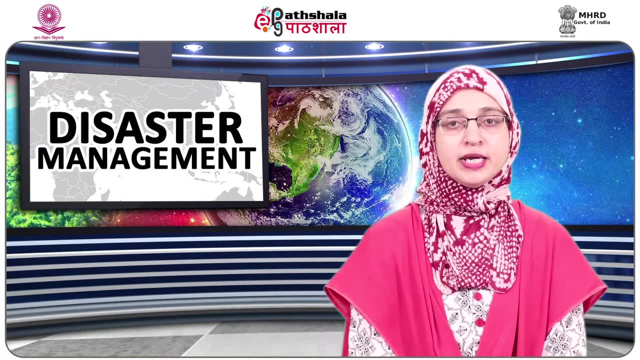 Declaration. Drought Declaration initiates the formal government response to drought situation. Based on drought declaration, the relief assistance and other supports are provided to the affected people. Traditionally, the revenue department heads, mainly the collector, recommends declaration of drought based on the crop production inputs obtained from revenue department officials. 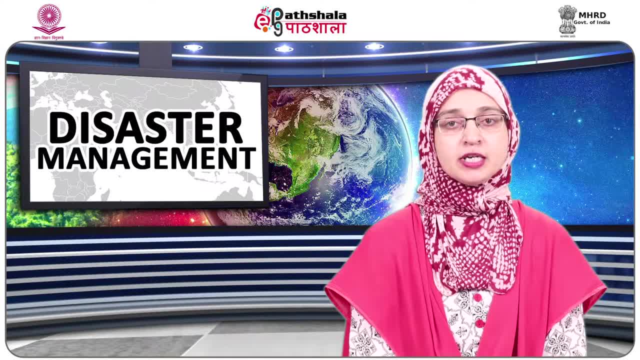 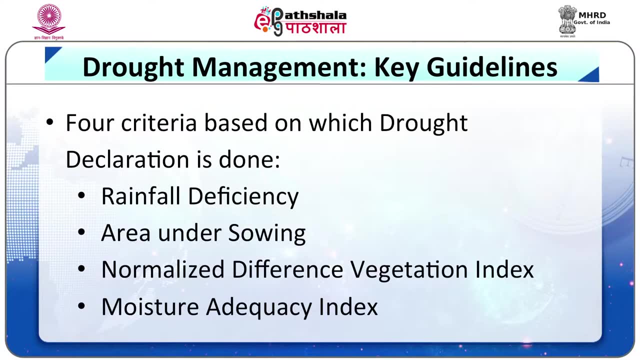 present in the drought affected areas, that is, typically villages. The final data on crop production is usually available in the month of December for Kharif Krop and in March for Rabi Krop. There are four criteria based on which drought declaration is done. 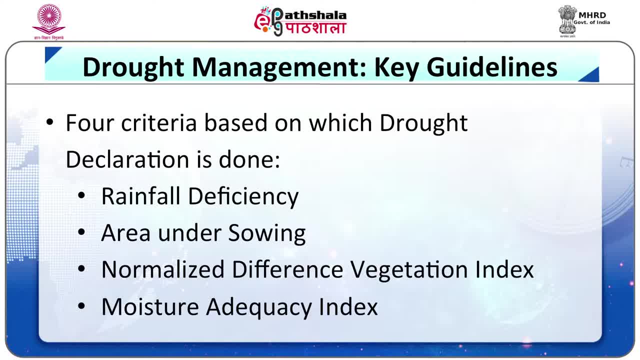 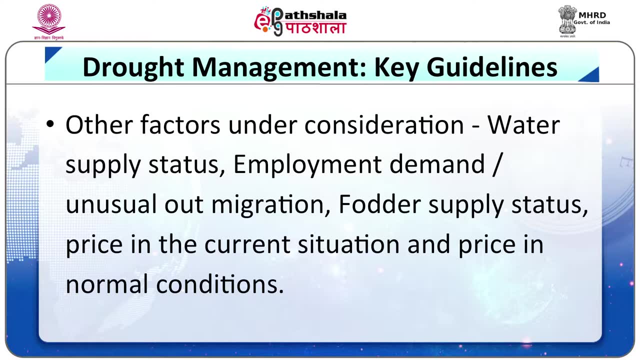 Number A: rainfall deficiency. Number B- area under sowing. Number C- normalized difference vegetation index. Number D- moisture adequacy index. The other factors under consideration are number 1, water supply status. Number 2, employment demand. that is unusual out my 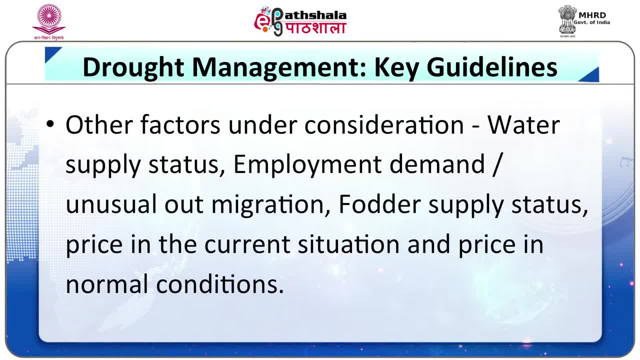 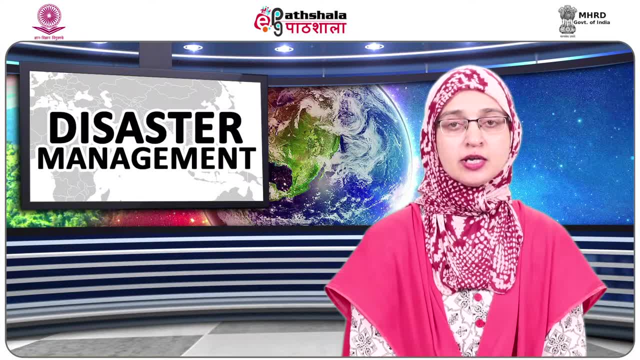 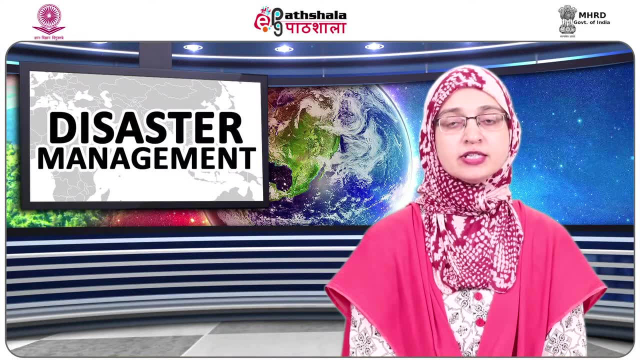 house. there is reclamation Number 3, fodder supply ratio: price in the current situation and price in normal conditions. Number 4, agricultural and non agricultural wage rates in the current situation compared to price in normal conditions. Number 5, supply of. 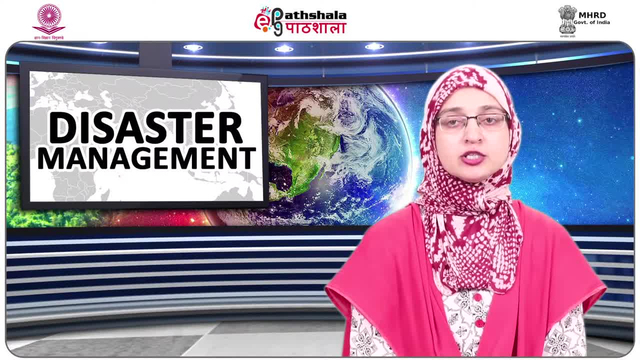 food, grains and essential commodities in the current situation compared to price in normal conditions. Number 6, Food prices which are used in��다 environment: Number 7,. cote Number 8,. apple: Number 19.. Number 10.. Number 31.. Number woe Number. 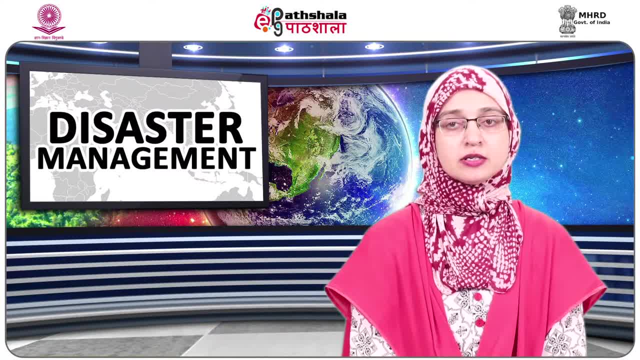 23. Once upon a time football. Once upon a time football. Once the drought declaration is done, the drought response and relief process takes over. Due to the multifaceted nature of droughts, the response involves an amalgamation of different 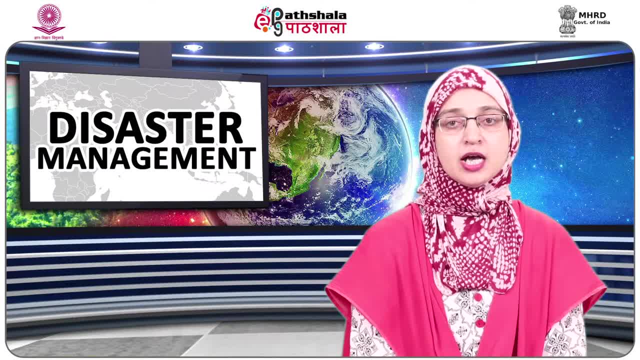 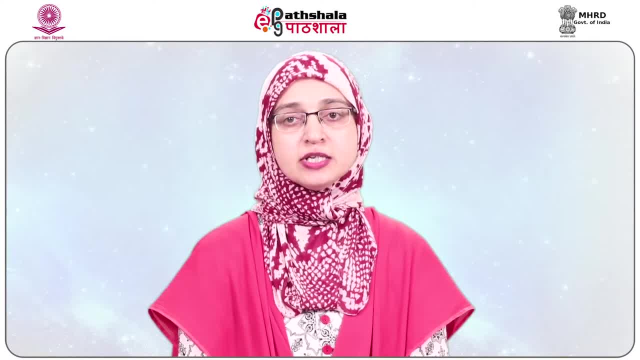 activities from different but interlinked sectors and involves several agencies. The measures typically employed include number one contingency crop planning. It aims to provide other cropping options to farmers which are drought resistant. It also provides alternate cropping strategies and mid-season correction and crop life-saving. 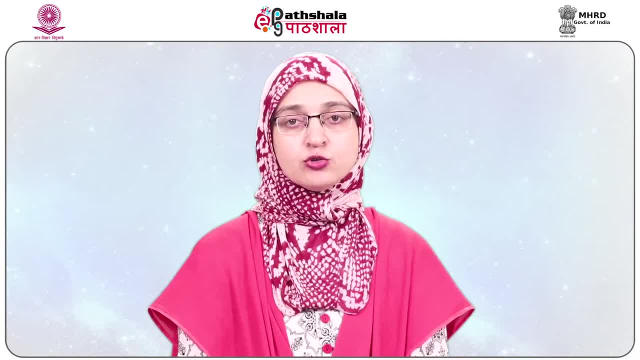 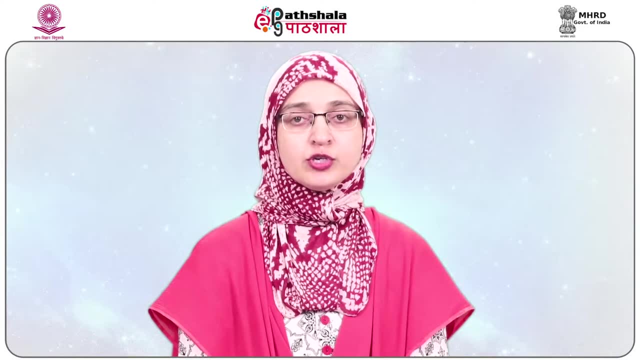 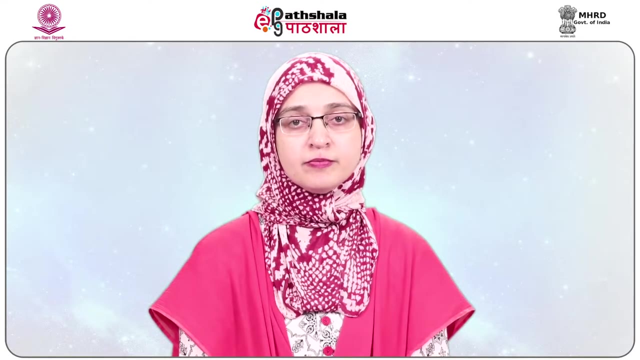 measures. Number two: relief employment. Due to drought induced employment loss, the government arranges for relief employment programs with cash and food grain assistance. Number three: water resource management- alternate sourcing of water. This includes diversified measures for ensuring the availability of and access to water. 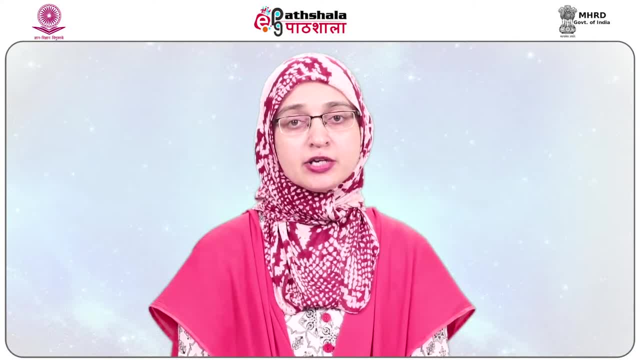 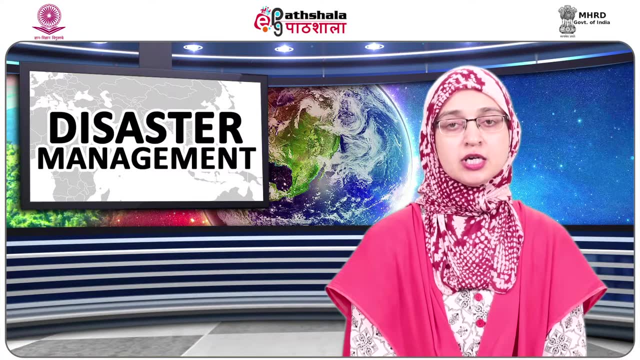 Measures such as augmentation of water supply, rationing, water use, efficient utilization and management of water resources are key elements under this initiative. Number four: food security. To maintain the food security status, special provisions to provide food, as well as checks and balances. 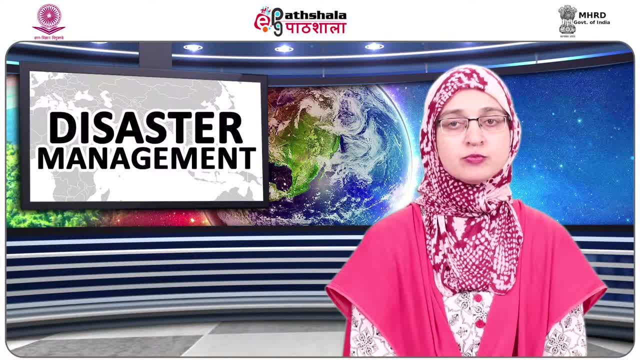 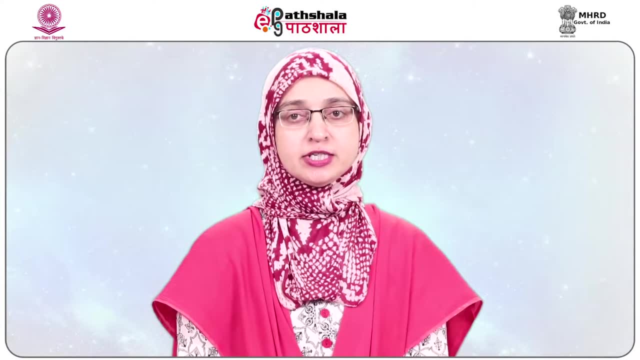 To ensure nutrition aspects of food are introduced. Often, wages in the employment programs are paid in the form of food grains to ensure availability and access to food and also minimize any chances of inflation. Number five: gratuitous assistance. This is considered as the assistance in the form of cash or food grains to people who 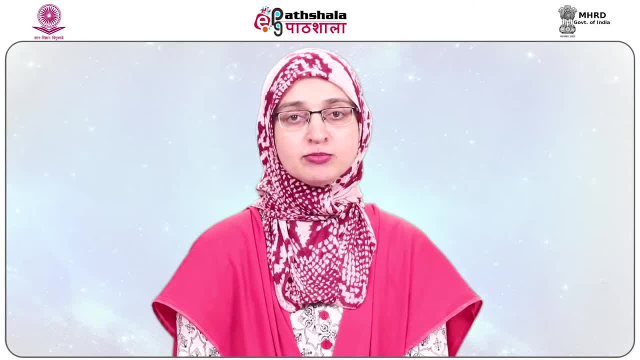 might not be able to participate in the relief employment programs or who are in the category of dependents. Number six: relief through tax waivers and concessions. The objective of this kind of assistance is to help people meet their basic entitlements. The tax waiver and concession amounts are decided based on the needs of the affected. 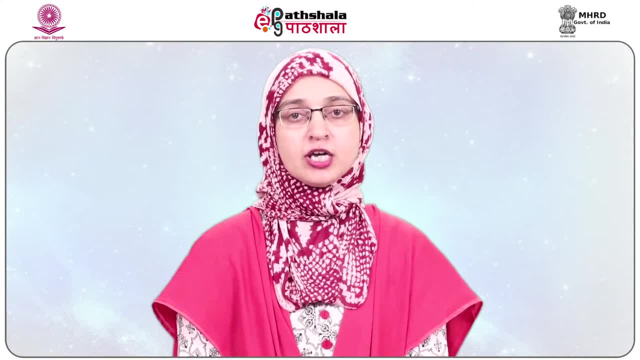 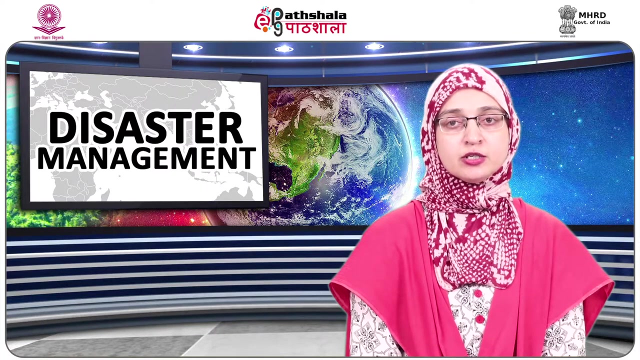 and the fiscal implications of such a relief to the government. Number seven cattle camps and fodder supply. Through such interventions the government provides necessary assistance to farmer in protecting their cattle by providing necessary assistance for their fodder, feed and health. This is done to discourage distressed selling of cattle, which is an important asset to farmers. 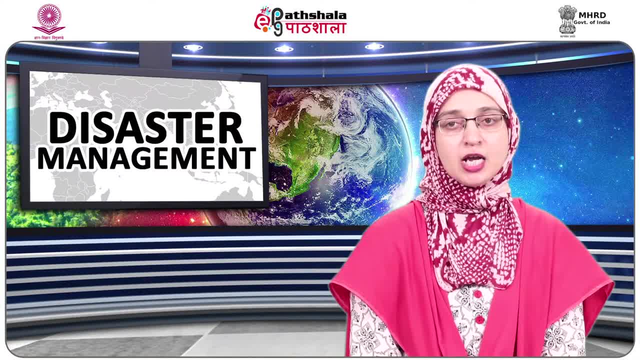 Number eight: health and hygiene. This kind of assistance helps maintain the health and hygiene of the affected. It includes measures to improve drinking water quality, disinfect drinking water sources, conducting regular surveillance, etc. in drought affected areas. Number eight: health and hygiene. 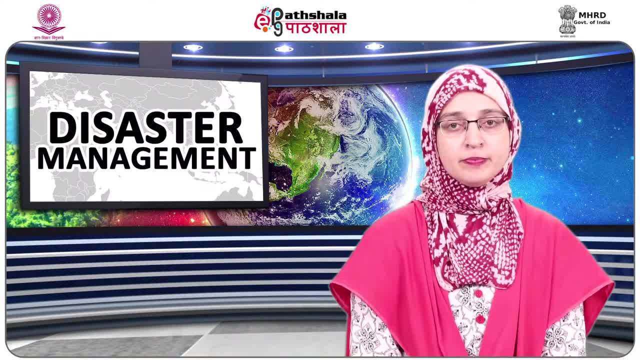 This includes measures to improve drinking water quality, disinfect drinking water sources, conducting regular surveillance, etc. in drought affected areas. This includes measures to improve drinking water quality, disinfect drinking water sources, conducting regular surveillance, etc. in drought affected areas. 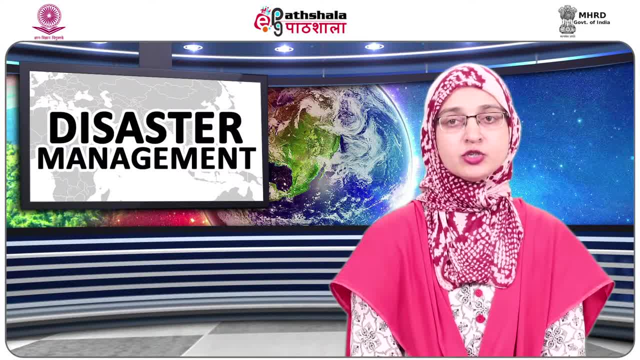 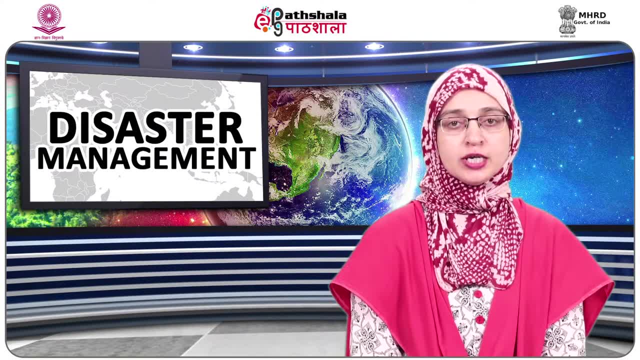 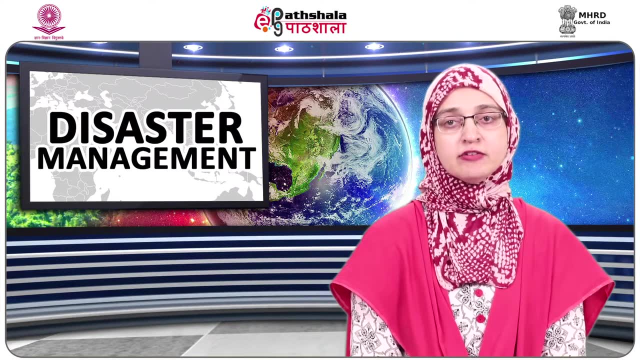 Number nine: financing relief expenditure. The Ministry of Finance releases fund releases. the Ministry of Finance releases funding from both CRF and NCCF to affected states based on set guidelines. This fund is utilized to perform the different activities and provide and provide financial assistance to the affected. 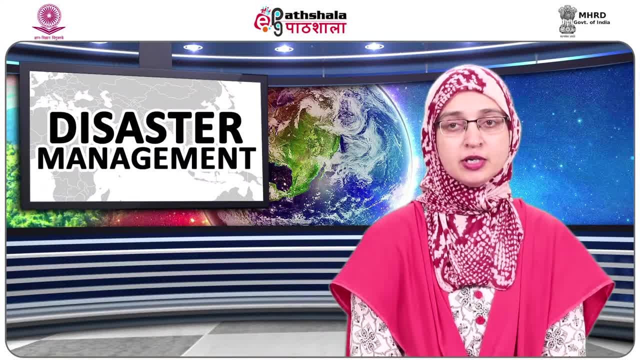 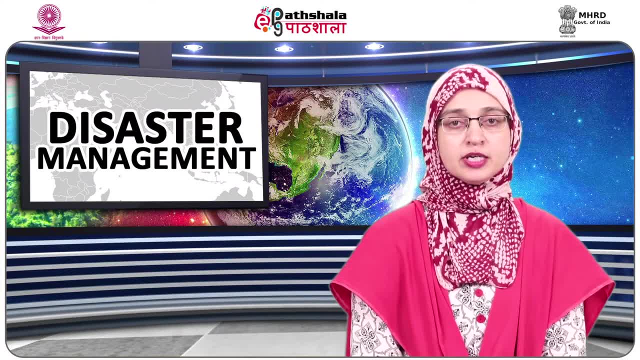 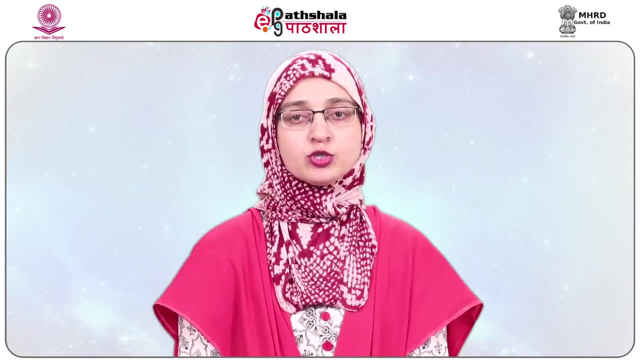 Number 10, information management and media coordination. This plays a crucial role In drought management and information dissemination to the affected community. Number D: drought prevention and mitigation measures. Multiple measures are proposed to mitigate and prevent the impact of droughts, which include: 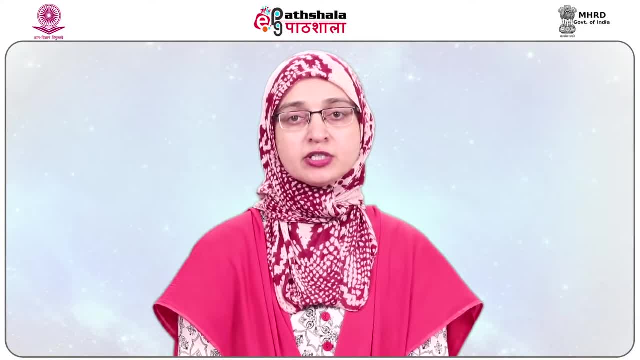 but are not linked to number one: water harvesting and conservation. It includes both technical and traditional methods. Technical processes include development of percolation tanks, Injection valves, Injection valves, Injection valves, Farm ponds, contour trenching, etc. Traditional methods include promotion of tankars, cones, boulis, spring water harvesting, etc. 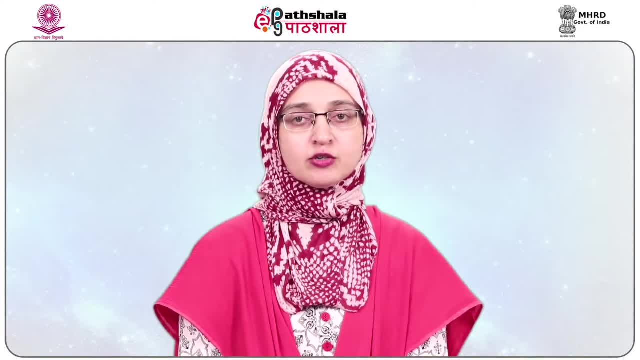 Number two: utilization of water saving technologies. Dip and sprinkle irrigation system. Dip and sprinkler irrigation system. Tip and Sprinkler irrigation system. Picking and sprinkler irrigation systems. Tip and Sprickler irrigation systems. Нumber three: long-term irrigation management. 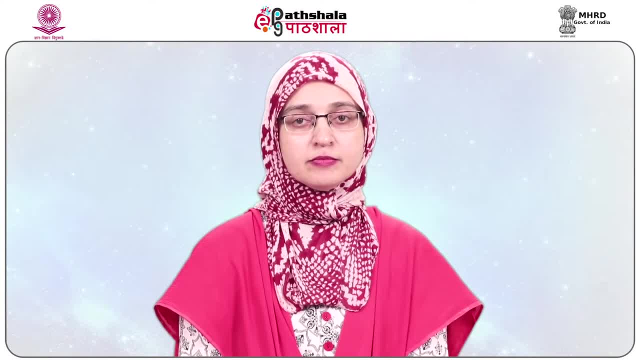 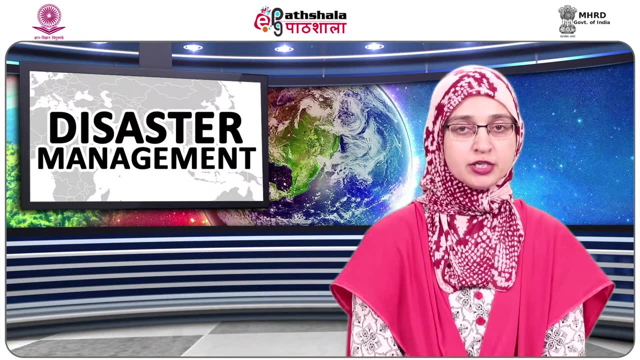 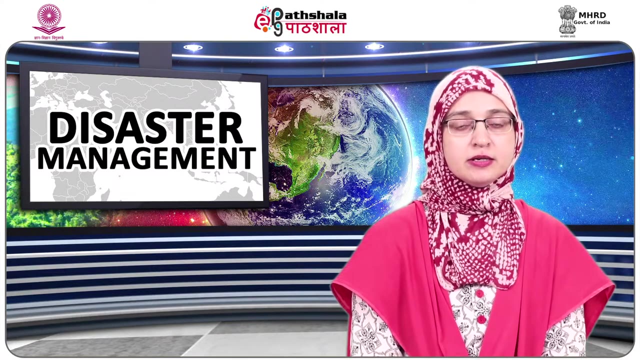 Borake soil management. Number for aphorestation, Bona, bioregulation and water conservation. Number 5, crop insurance. Number 6, community participation in drought mitigation. It includes: number A- built on micro level experiences. Number B- innovative community based institutions. 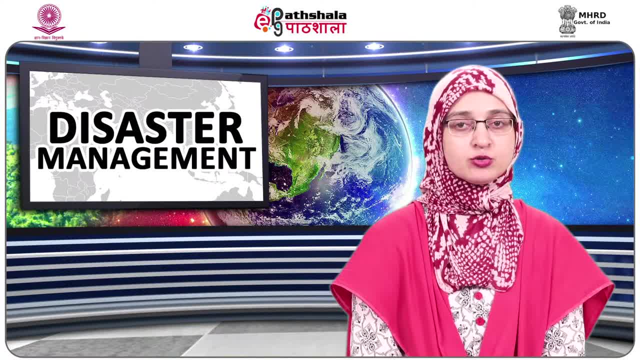 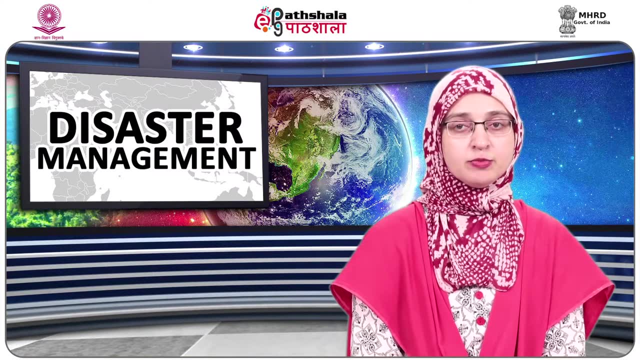 Number C: organized community based consultations through gram sabha. Number D: strengthened self-help groups. Number E: empowering panchayati raj institutions. And number 7, adaptation to climate variability. Drought mitigation programs are currently underway. that includes number A. 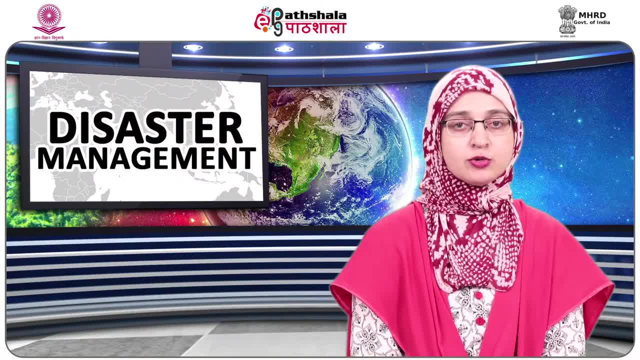 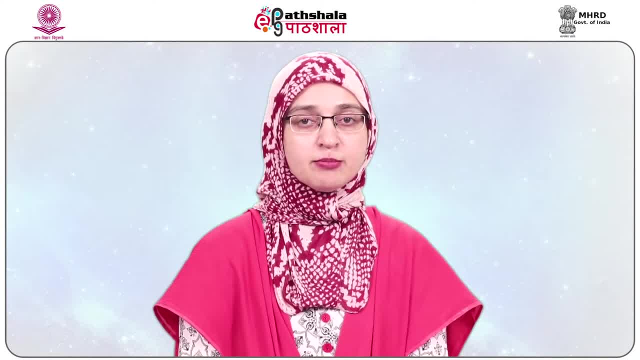 the national rain fed areas authority aims to address the issues of drought in the long term perspective. Number B: drought prone areas program. Number C: desert development program. Number D: integrated watershed management program. Now E: capacity building measures. The NDMA guidelines provide detailed inputs on national training and capacity building measures. 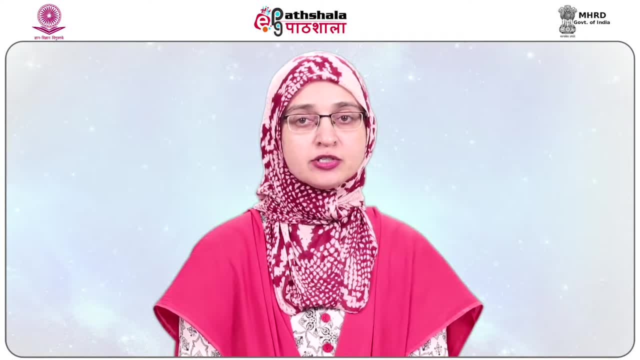 for drought management. It suggests training in drought management through identification of training needs, training of trainers, development of training manuals, training of professionals, strengthening training and research institutes, etc. Apart from such institutional measures, it also focuses on developing community awareness. 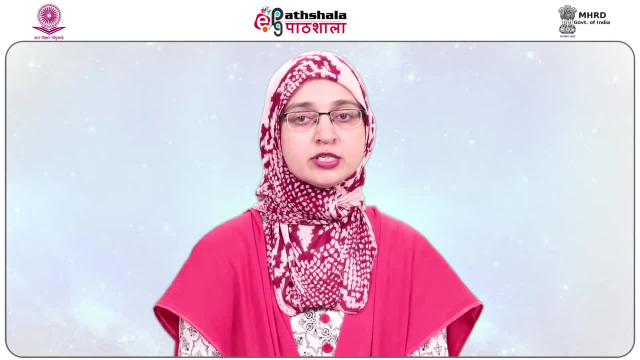 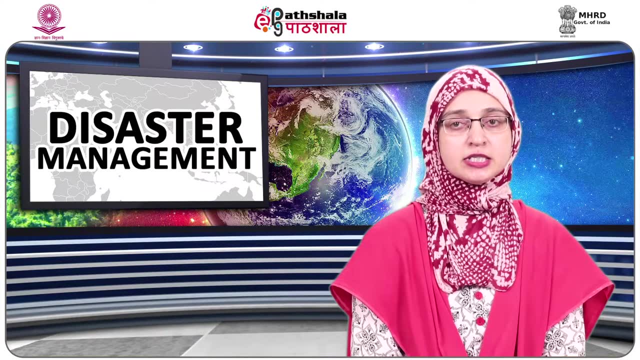 documentation and community participation for holistic development of capacity utilization. Now Marathwada case study. To illustrate the functioning of the guidelines mentioned above, the government intervention in Marathwada region is taken up as a case study. The Marathwada Agrarian Crisis, with Indume hobbyists crisis, is an odd one. 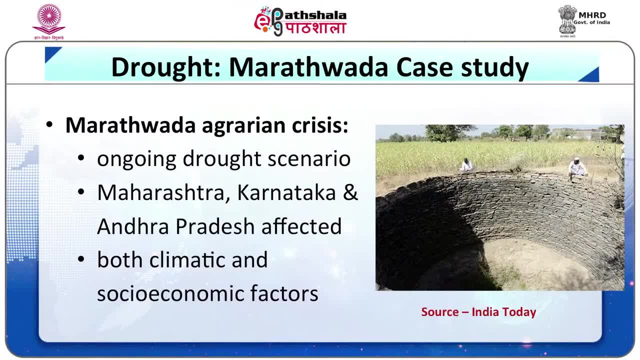 Nor is it the specific kind of study that should be introduced. As a consequence, the injured disabled and the injured don't have much to learn and large简idencelaration implementation is an ongoing drought scenario in which extensive area of Maharashtra, along with parts of Karnataka. 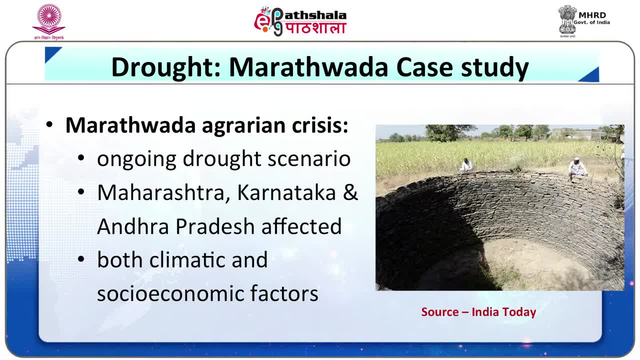 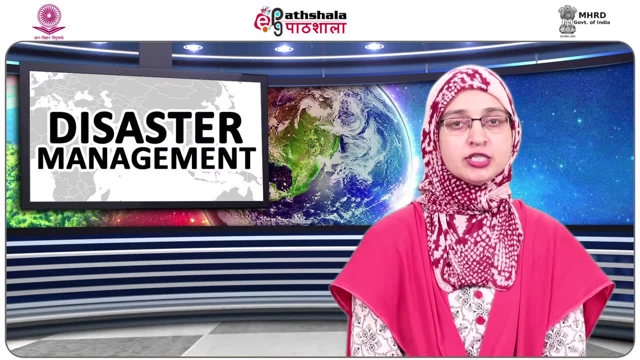 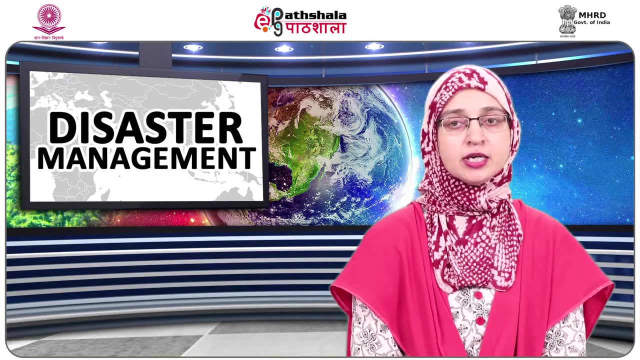 and Andhra Pradesh is affected. Both climatic and socio-economic factors are attributed to the ongoing crisis. Along with below average rainfall, changes in the cropping pattern, providing more importance to water-intensive cash crops like sugarcane and grapes is primarily blamed for the crisis. Allocation of more water to cash crops, depriving traditional water drought. 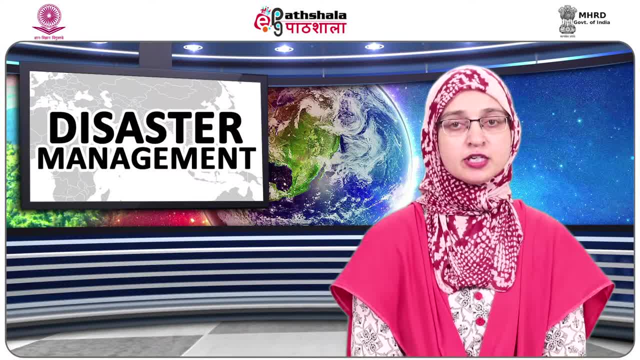 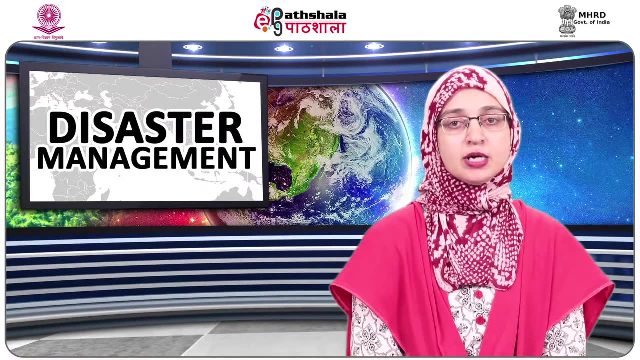 resistant crops, indiscriminate usage of limited surface water and groundwater, depletion of the groundwater level, large-scale diversion of water for industrial purposes have resulted in extreme shortage of water. To address the ongoing crisis, multi-prolonged strategy has been utilized by the 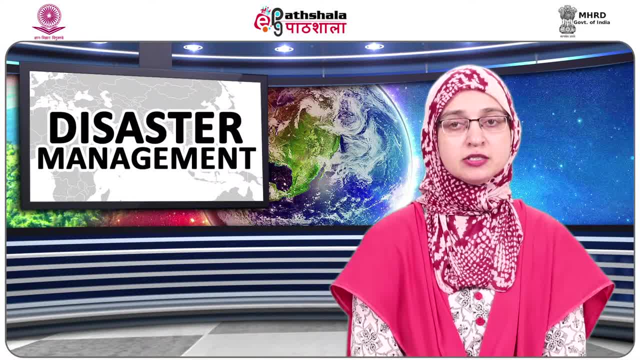 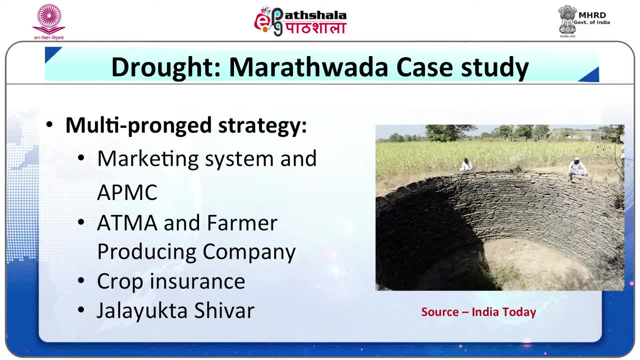 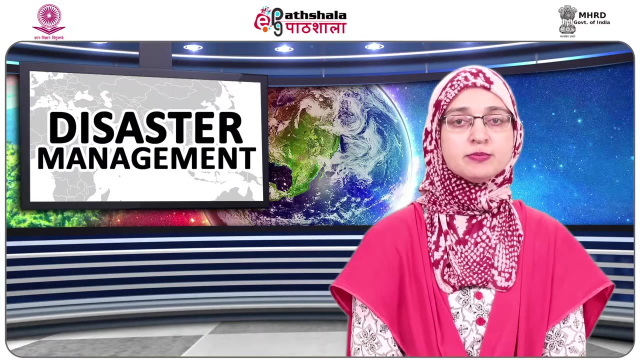 state government in association with Maharashtra Non-governmental agencies. Some of the key strategies include: 1. Marketing system and APMC To minimize better provide support systems to the agriculturalist and minimize the impact of middlemen. marketing systems are set up In such markets. the minimum. 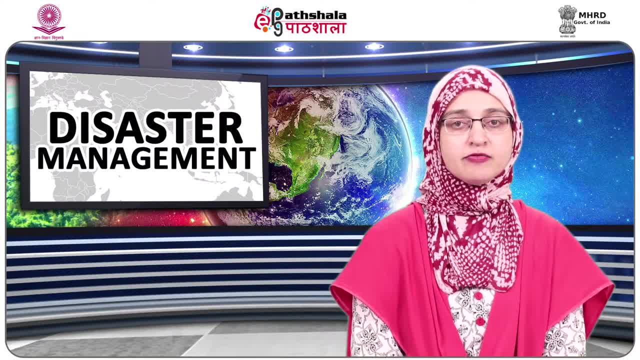 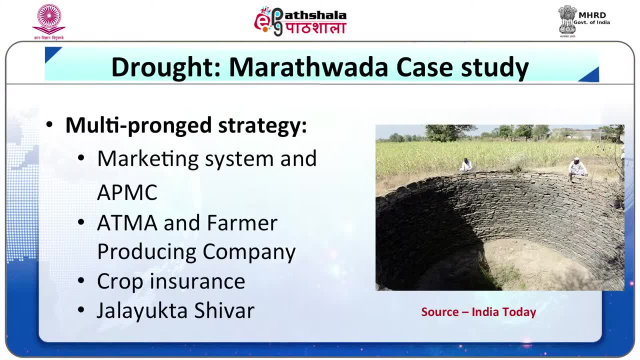 support price for the product is guaranteed, which helps the farmers in not getting underpaid. 2. A TMA and Pharma producing company. The main functions of an institution like ATMA, in collaboration with the agriculture department, is to provide technological support, seeds, fertilizers and 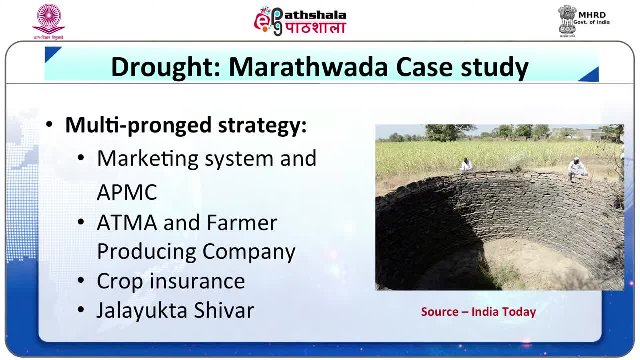 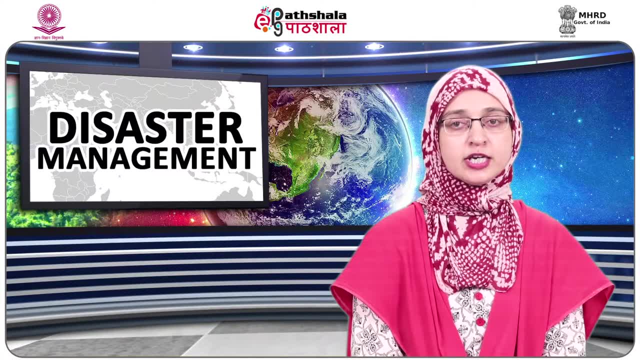 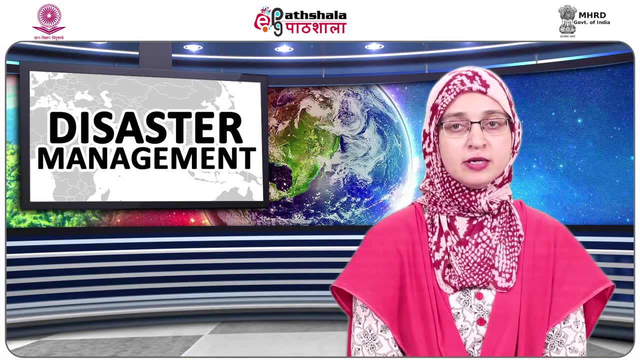 tools and instruments for mechanization of farming at subsidized rates, organized demonstrations and training programs. It also aims to facilitate formation of pharma producing companies of 15 to 20 members, based on competition. 3. A Common Farming Practices. These VPCs will function as a collective unit. 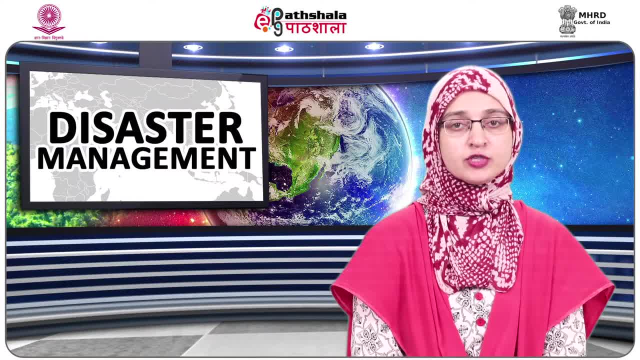 It will give the farmers better bargaining power in terms of sale of product and purchase of raw material. Also, it will lower transport and allied expenses and facilitate in collective training and skills development program. Also, demonstrations are arranged for farmers where particular way of farming is done and the 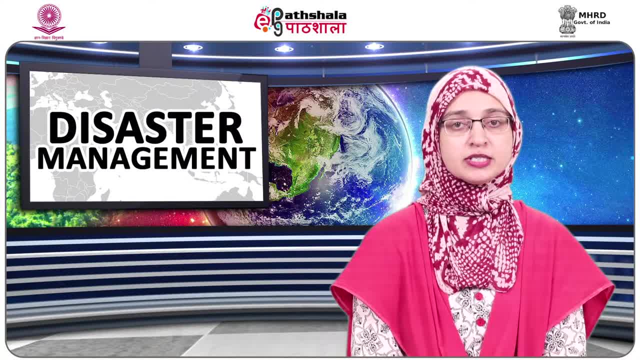 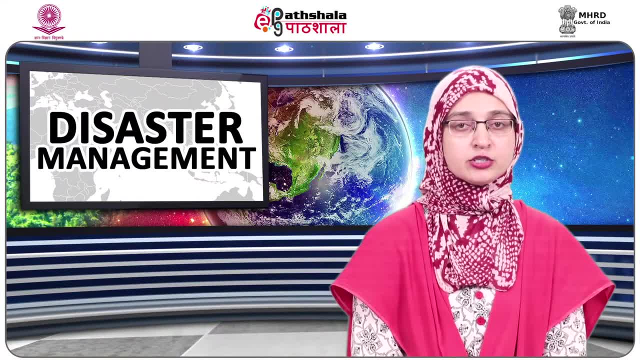 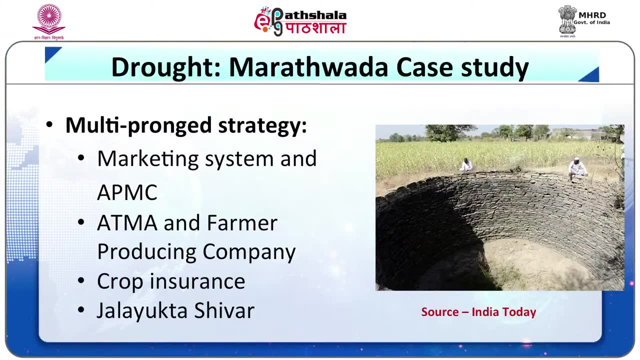 profits in terms of Yields were shown to motivate farmers to savoir more about farming activity. in cultivating the same crops. the same way, Promotion of drought-resistant crop cultivation, mixed crop cultivation and required technologies are being promoted through such initiative. Number three: crop insurance. Crop insurance is being promoted as one of the most important risk. 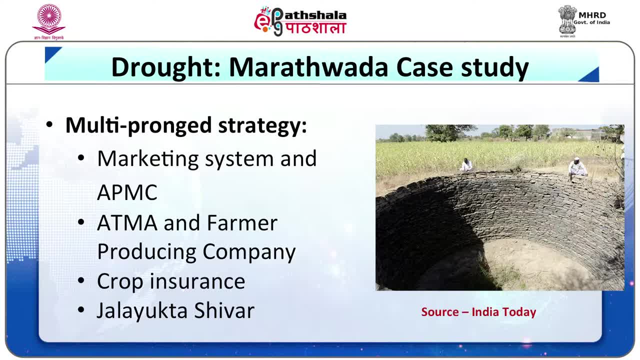 transfer mechanism. Number four: Jala Yukta Shiva. This is an integrated water resource management project implemented by the government Under the umbrella of the project: deepening and widening of streams, construction of cement and earthen stop dams, work on Nannulas and digging. 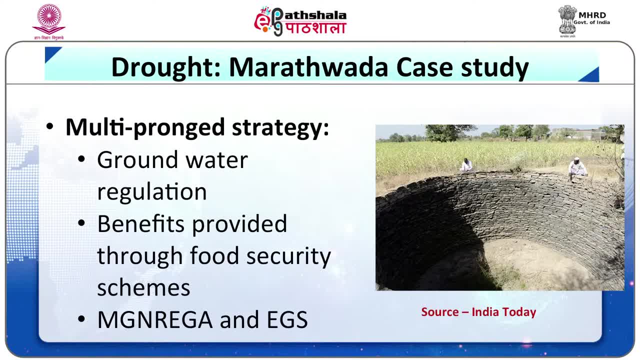 of farm ponds, etc. are under progress. Number fifth groundwater regulation: Drying of bore wells is a serious concern. Government circulars on bore well depth have been issued to address this. Number six benefits provided through PDS system and other food security schemes in drought affected. 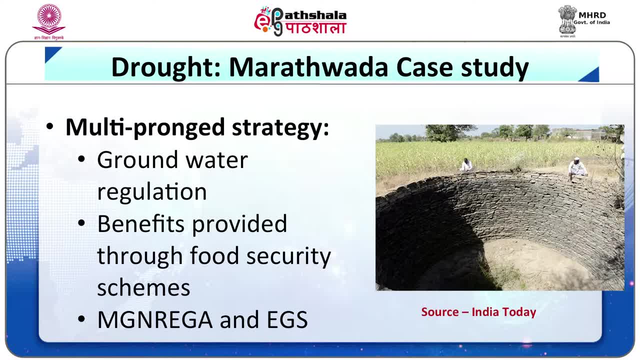 area. As the area is drought affected, extra provisions under PDS system for ration card holders have been arranged, which is very helpful. Midday meal scheme is also functional in most areas to maintain nutritional status among children: Number seven, Manrega and employment. 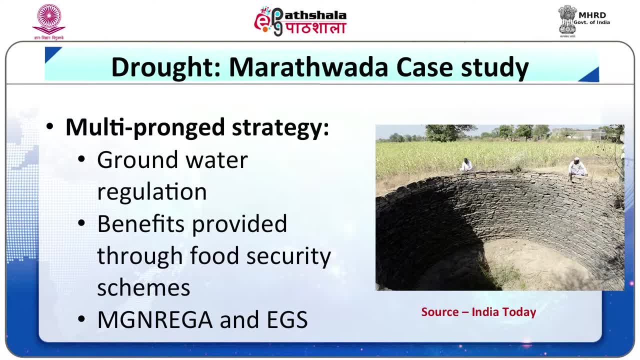 guarantee scheme that is, EEG. In most of the villages, Manrega and EEG schemes are helping in providing economic support to deal with the agrarian crisis. The registered people are provided employment for certain duration of time every year, guaranteeing the income, Also utilizing Manrega and EEG administration. 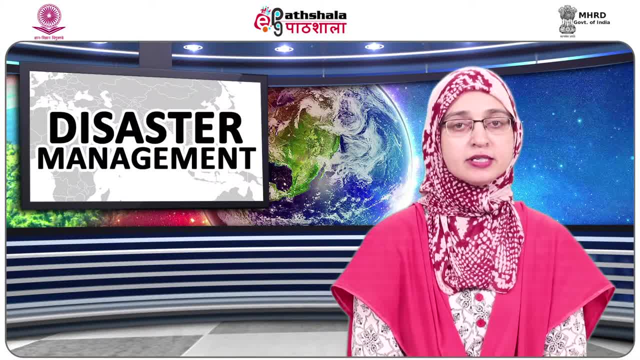 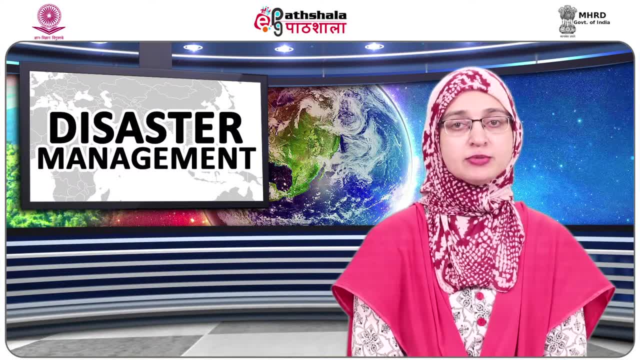 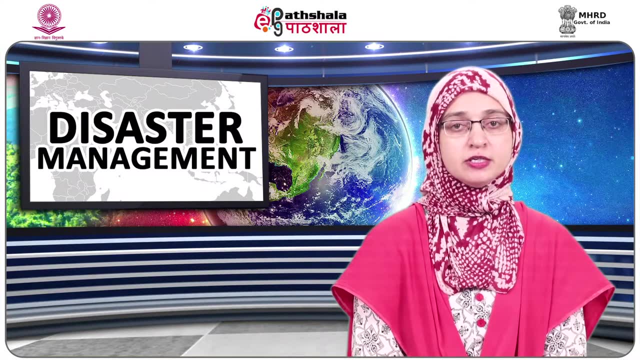 is developing water resources and implementing mechanisms to improve drought resilience. This is merge with the Jalayukta Shiva scheme, which aims at integrated management of water resources. Number eight: seeds, fertilizers and other subsidies. Seed's, fertilizers and tools are available at subsidize rates under various schemes and 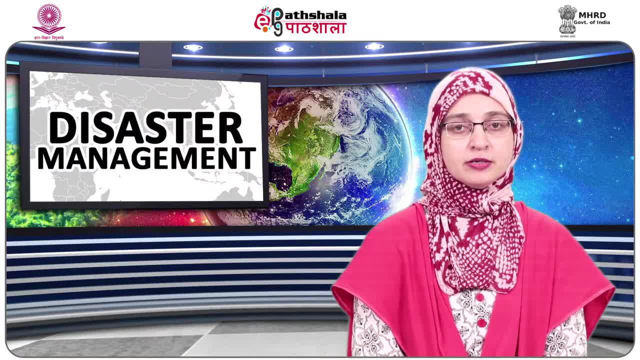 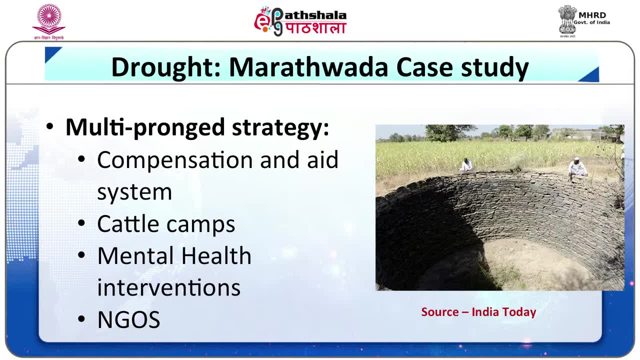 there is no upper limit on the amount that can be requested. Number nine: compensation and aid system: Government initiated compensations and aids to the affected have been issued should Based on the official criteria on the loss of a specified portion of agricultural produce. 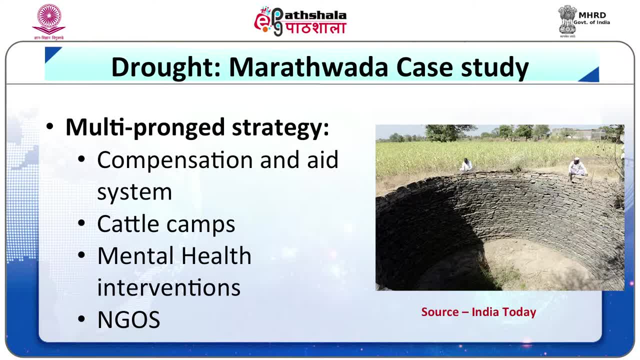 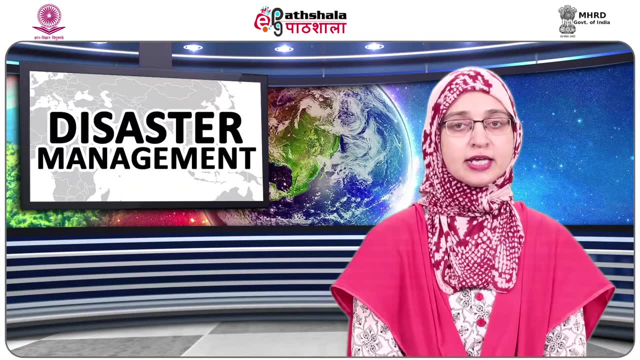 compensation is provided by the government after inspection by ground staff. 10. Cattle camps. Cattle camps are set up in many areas in the affected region to assist the affected farmers maintain their livestock. To maintain the cattle camps, government provides subsidies to the cattle camp owners to arrange for fodder and other. 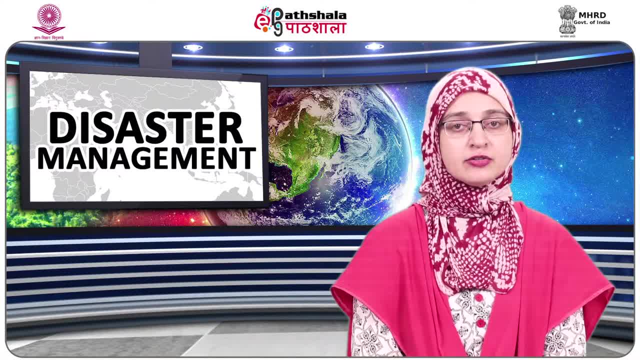 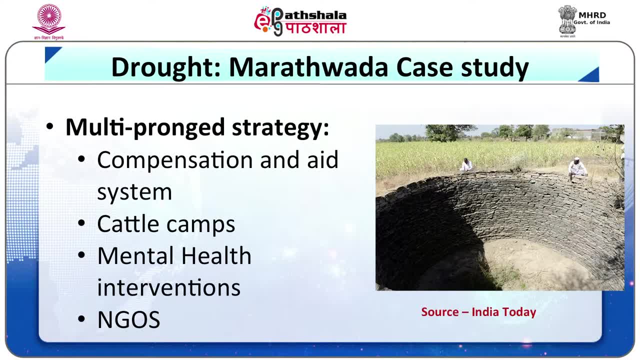 provisions for the cattle. The farmers can shelter their livestock in the cattle camps during the drought period. 11. Mental health interventions. Due to the large number of suicide incidences, the state government has launched integrated mental health interventions under the flagship of Prerna project, Under the project people. 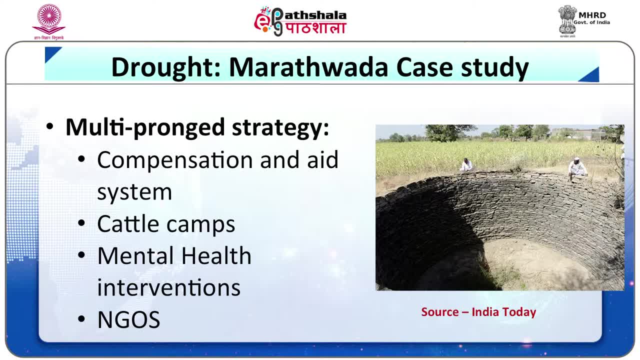 affected by mental health stressors are eradicated. 12. Asha workers: Asha workers in different villages act as Prerna workers. The guidelines for Prerna workers include: 1. Identification of farmers displaying symptoms of depression and anxiety. 2. Provide guidance on how to address the stressors. 3. Steps to avoid people. 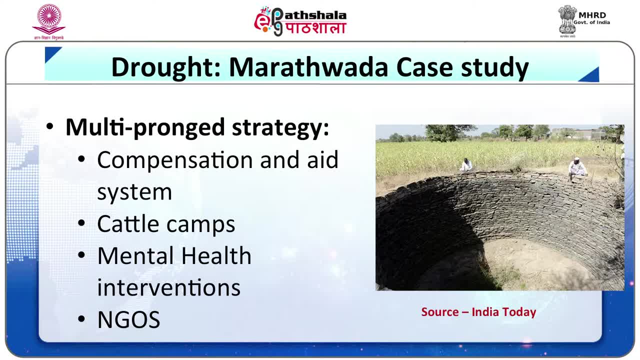 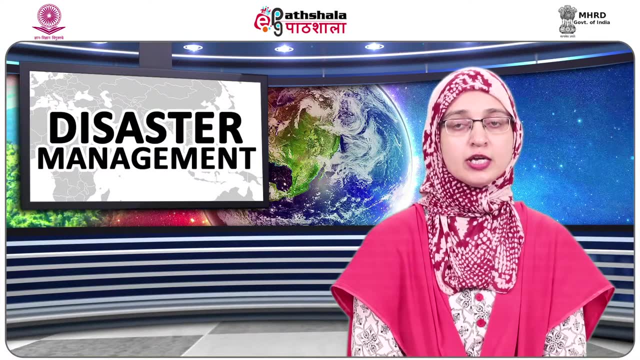 from committing suicide. When the village level Prerna worker is unable to address the issues, the person is directed to the sub-center where further care is provided to the individual. In cases where the issues cannot be addressed at the sub-center level, it is forwarded to the PSC and forwarded, depending on the severity. 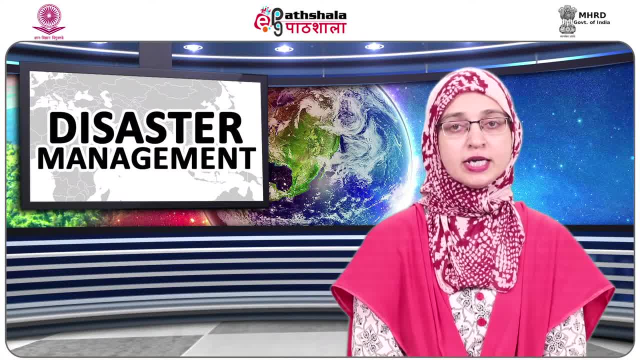 of the case. Additionally, schemes to provide health care and prevent economic distress occurring from health care expenses are introduced. Drug de-addiction programs are also introduced to promote well-being to the farmers. 12. Drug de-addiction programs. Drug de-addiction programs are also introduced to promote well-being. 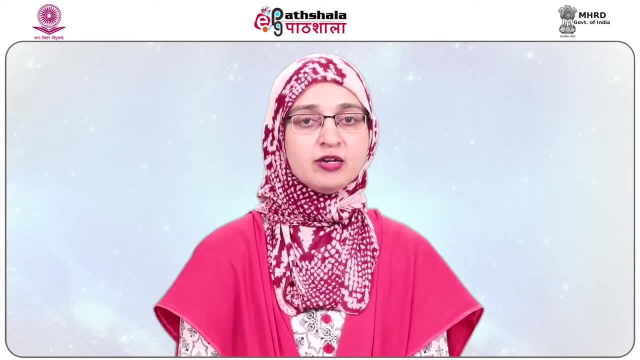 to the farmers. 12. Drug de-addiction programs. Drug de-addiction programs are also introduced to promote well-being of the farmers, Thus utilizing multiple social schemes and dedicated mental health intervention is developed to provide psychosocial support in the affected region. 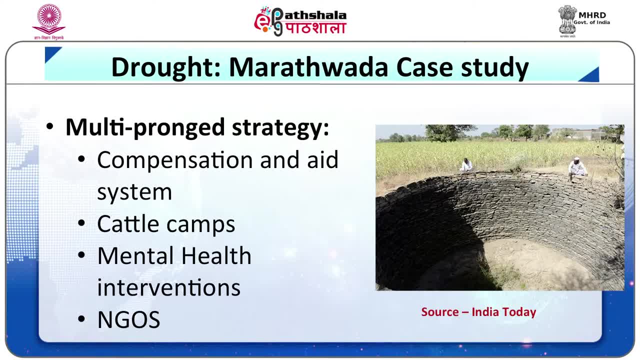 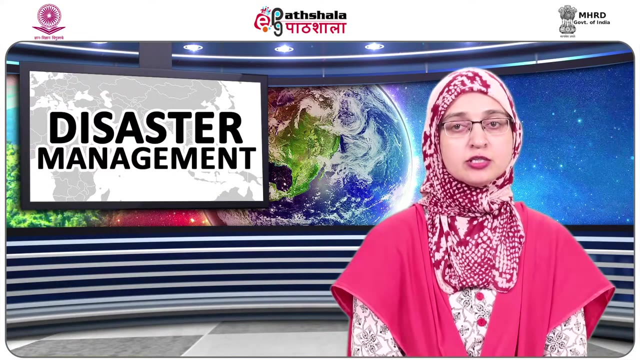 12. NGOs: Many NGOs have intervened to address the issue of promoting water resource management techniques and awareness generation. Through an effective partnership with governmental and state agencies, the government has been able to develop and implement a comprehensive plan to address the issue. 13. Drought: Drought is a slow-onset disaster which evolves over months and years. 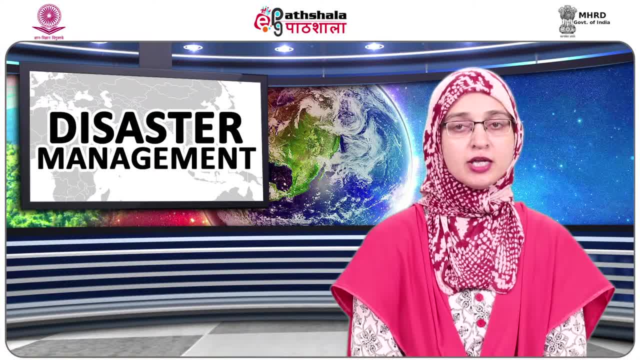 14. There are both environmental and anthropogenic factors causing droughts. 15. There are four broad categories of droughts: 16. Meteorological drought. 17. Hydrological drought. 18. Agricultural drought. 19. Environmental and anthropogenic drought. 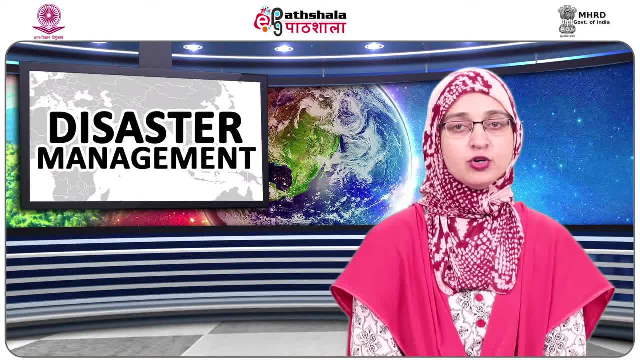 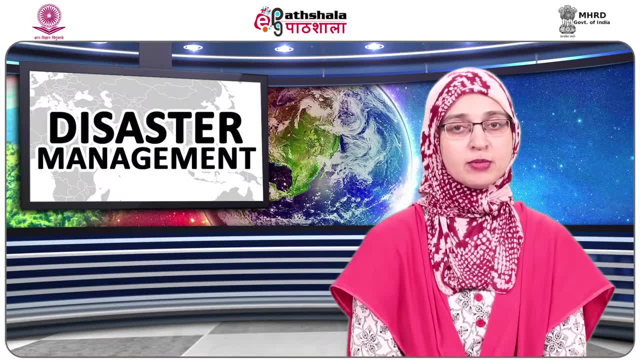 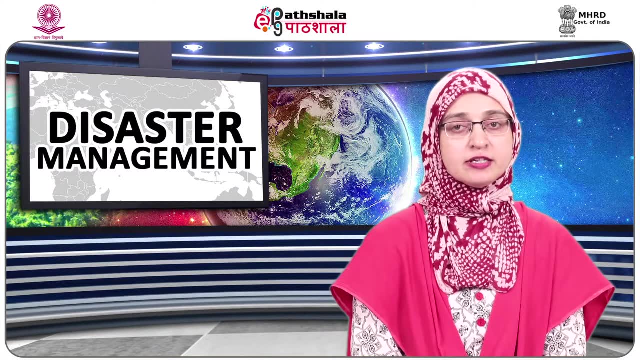 20. Natural drought and socio-economic drought. 21. Famine is a severe scenario where extreme scarcity of food is experienced, leading to mass malnutrition, starvation and increased mortality and epidemic scare. 22. Desertification results in extensive degradation of productive lands, loss of water bodies. 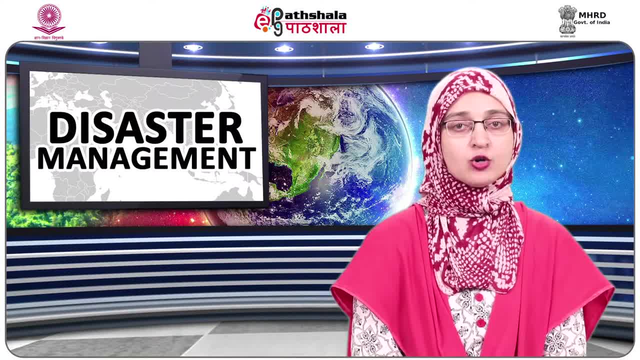 flora and fauna. 23. Drought impacts are of socio-economic and environmental in nature. 24. Drought occurred in almost all parts of the world till early 20th century. 25. India is highly prone to drought due to dependence on monsoon rains for agriculture. 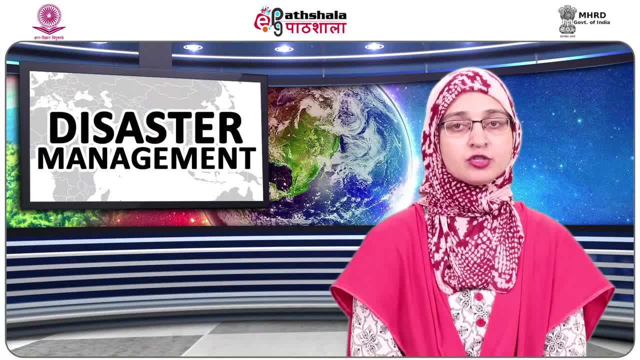 26. Famine commission, formed in 1880, was the first formal initiative for drought management. 27. The nodal department for drought management is Department of Agriculture and Cooperation. 28. Ministry of Agriculture. 29. Government of Agriculture.